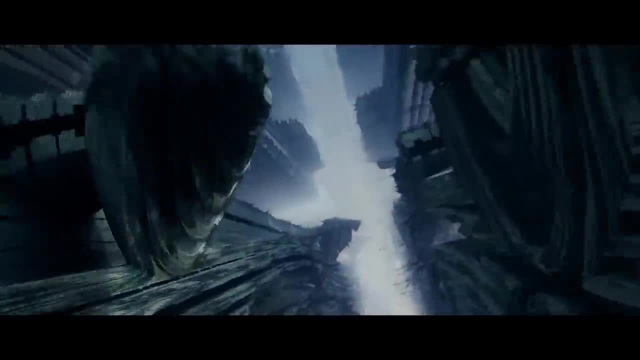 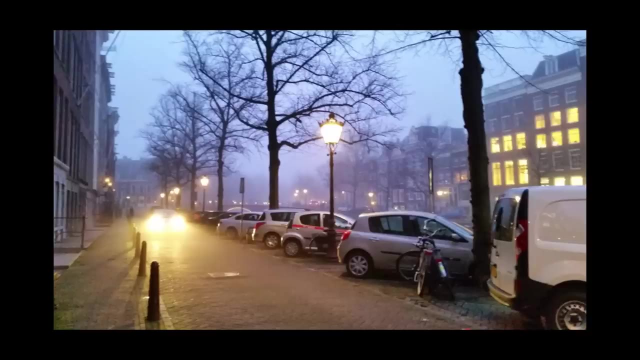 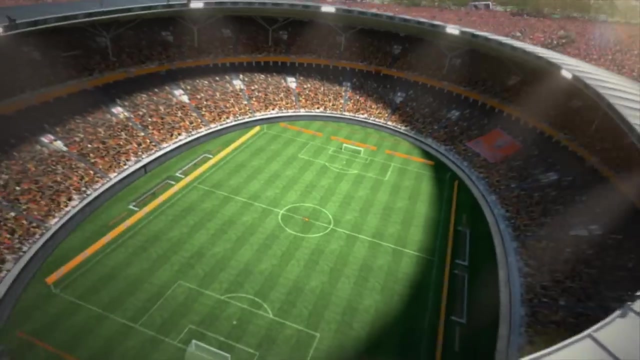 on sets etc. Also, I work for five years now for company Hectic Electric, which is based in Amsterdam, the Netherlands, on the lovely canals, which is a post facility- really great. we do lots of feature films and lots of TV commercials, mainly Dutch. 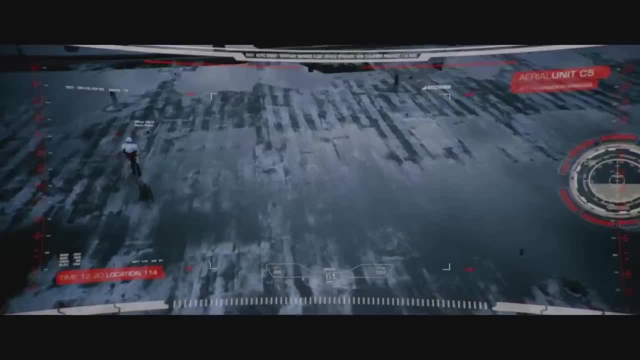 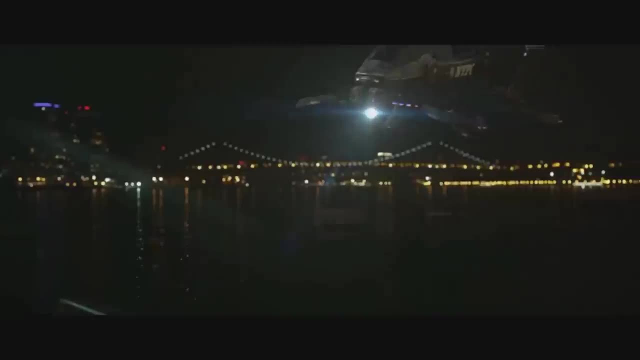 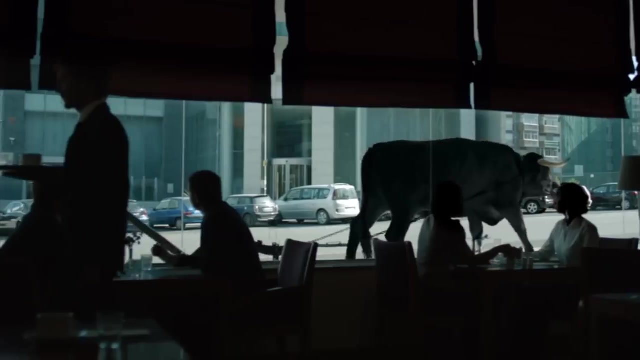 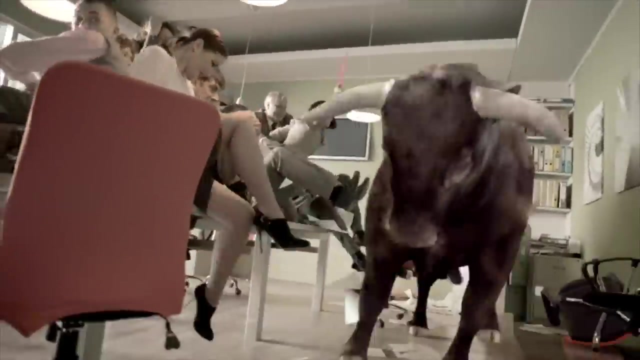 feature films, but we're also doing some, some stuff in in the USA, in America, and hectic electric is really good with stuff like real flow and effects and also the great fur pipeline. so especially for for the Netherlands, I think we do almost all the all the fur stuff. I've done a feature film which I 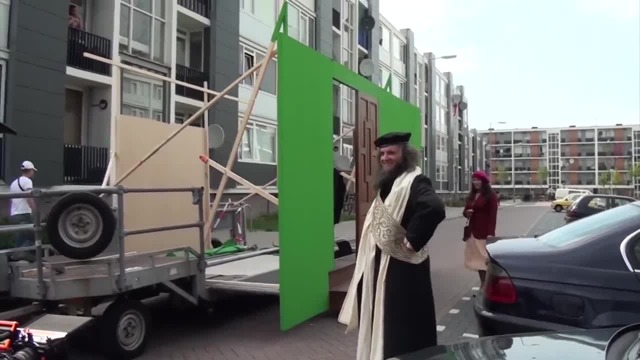 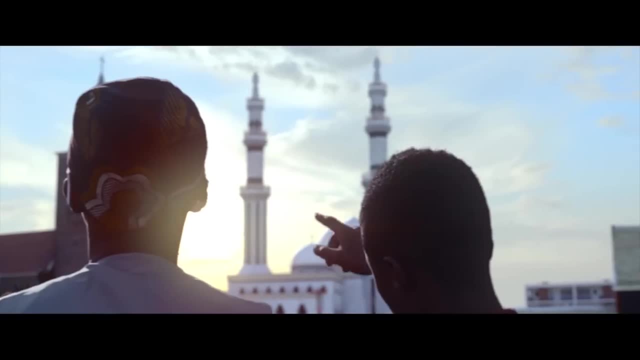 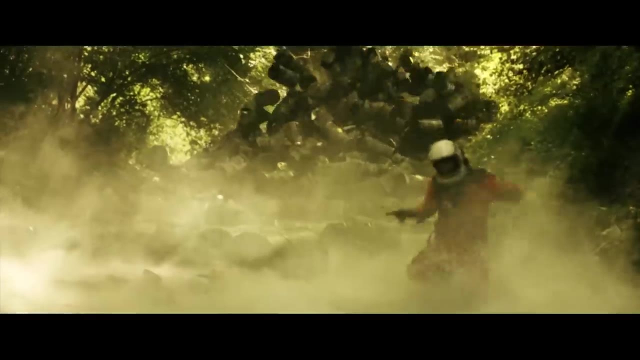 supervised about two years ago, called to be king or a coning from Catoa, which had like 850 effect shots and it was crazy and it was real fun. it had lots of completely CGI buildings that were moving and had a CG dragon or some kind of monster. rather lots of green screen, lots of matte. 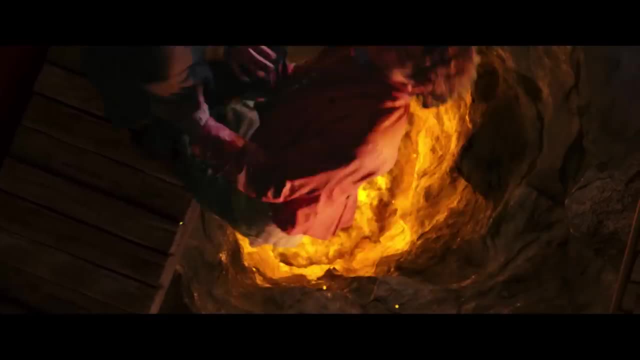 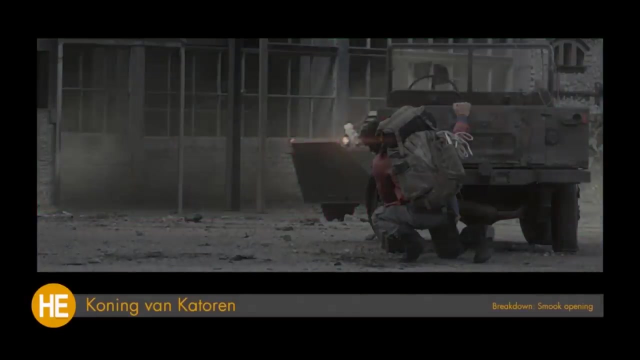 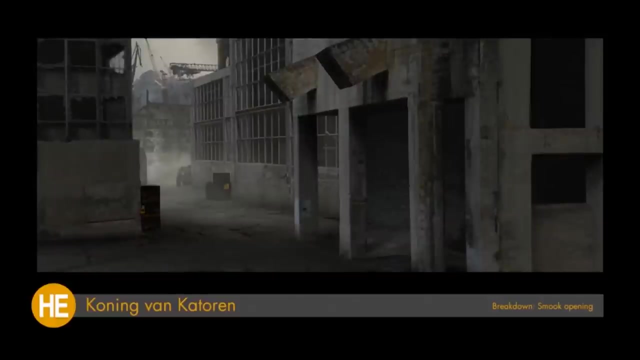 painting. it's real fun and great project to work on. I'm saying this because I want to let you know a little bit on the type of environment that I'm in, because I realized that lots of a fractal enthusiasts are maybe coming from a little bit more the programmer side of things. 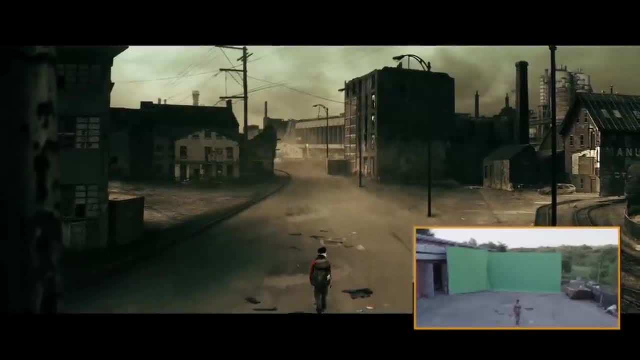 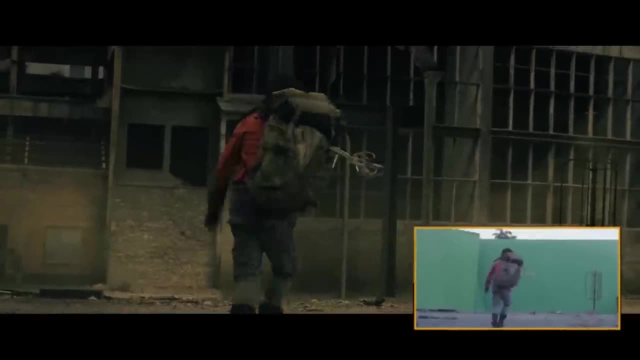 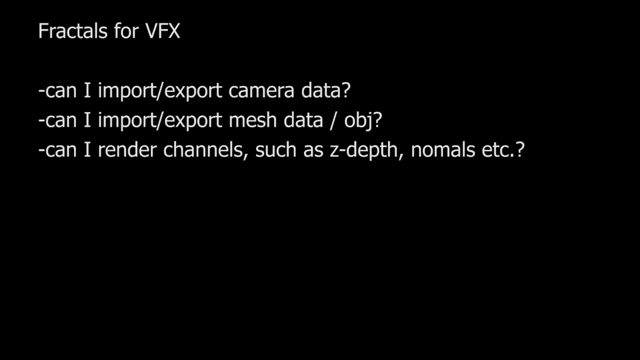 and I really want to hammer home that this is going to be about typical VFX pipeline stuff. can we use fractals in that? so how this is going to work is here. here's the questions that I that I get sometimes, and short answer to every question is actually no, no, you can't do this, no, you can't do that. but there's always a way around that, and so I'm gonna give you a quick answer to that, and we'll talk about that in a minute. I'll give you a quick answer to that in a minute. I'll give you a quick answer to that in a minute. 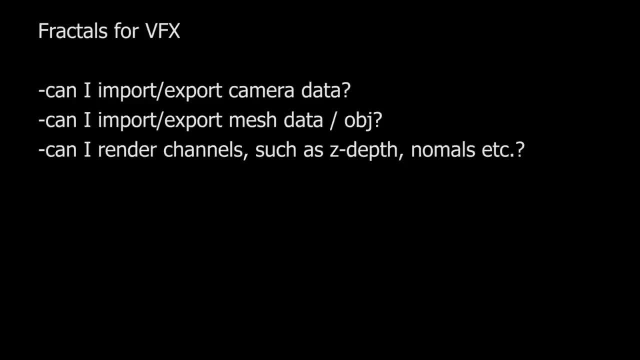 I'll give you a quick answer to that in a minute. first I'm going to give the short, short answer and then we'll explore the way around it. and one of the questions I get asked more most often- sorry- is: can I import or export camera data? and indeed the answer is no, you can't import or. 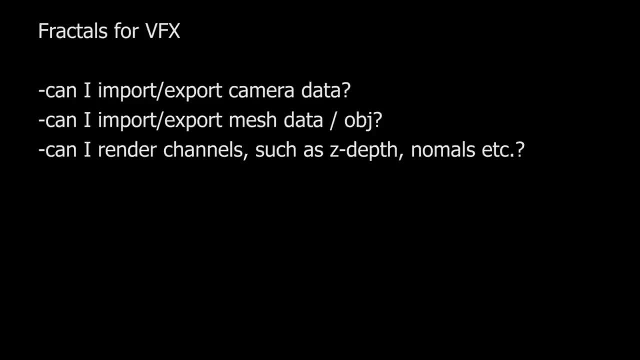 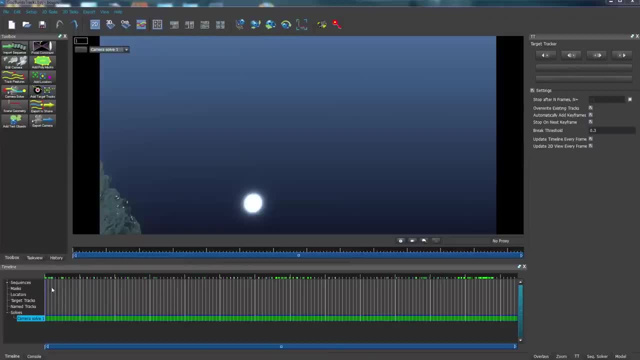 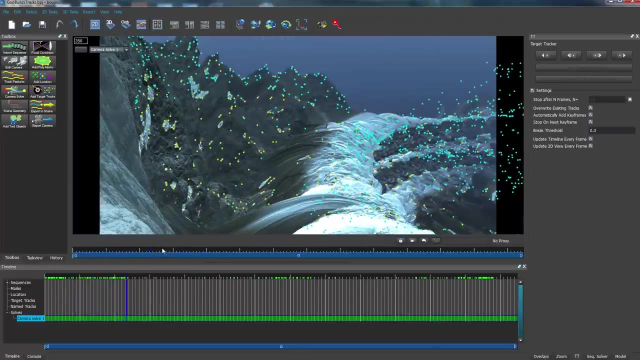 export camera data at all. there's no such function. there is no. there's no way to do that. that's the short answer. but then obviously there is a way to export camera data. the way to export camera data would be to render out your scene and then just to track it in boozhoo or synth eyes or PF track or whatever. 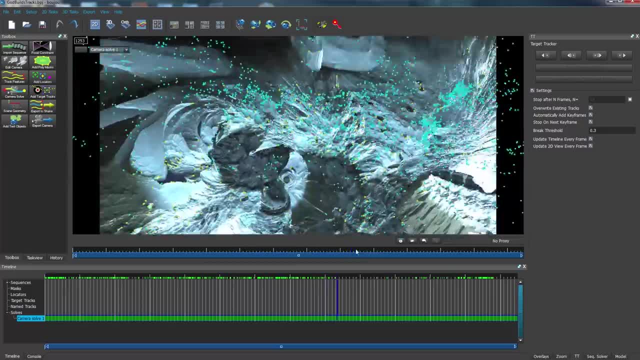 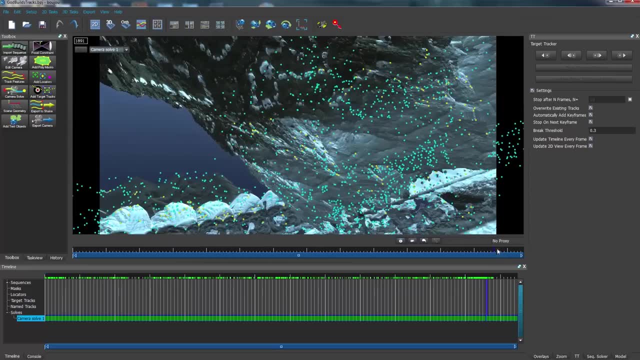 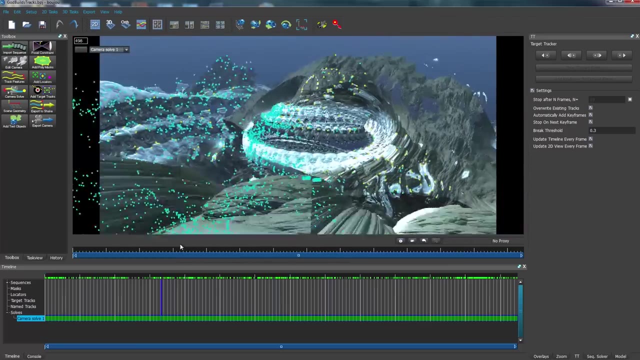 camera tracking software. you use because this? because this just completely works and it's very usable and a really great way to to to export your, your camera motion. but you would have to make your camera motion in inside the software, Mandel bulb 3d- and then by rendering it and tracking it, you can you. 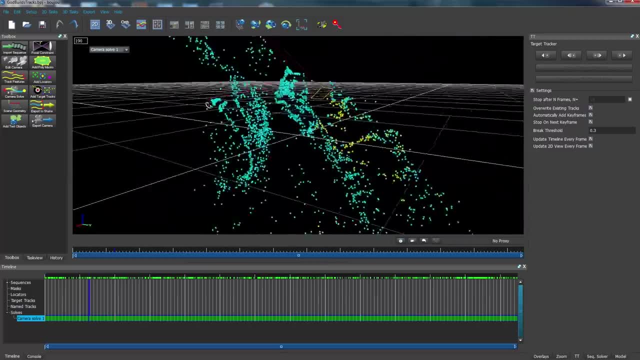 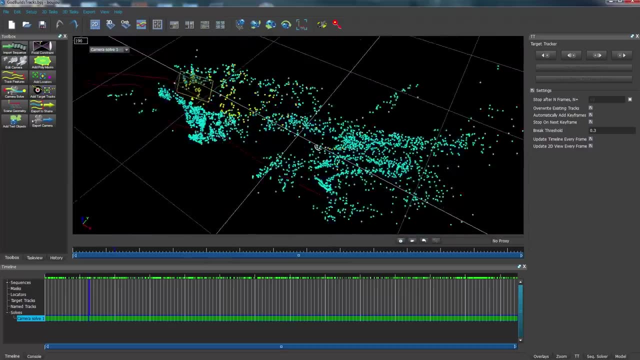 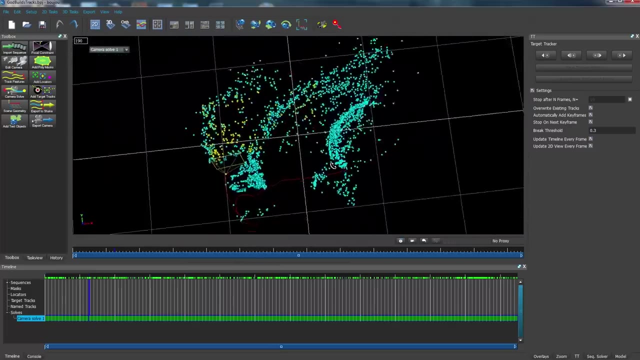 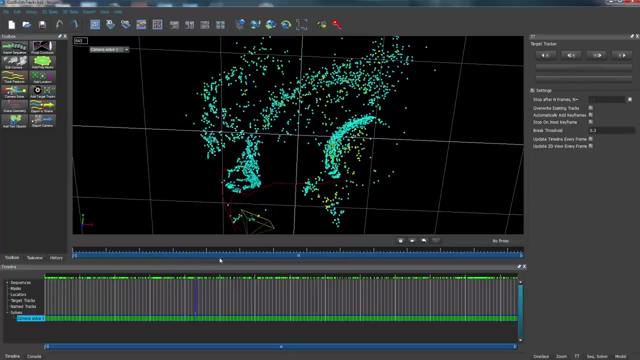 can export it. so this works, it works, it works well, and importing is really not possible. you can't really import an FBX or anything like that and I don't see any way you could actually even maybe by hands, like typing in the numbers, frame by frame. it Mandel Bulb is. 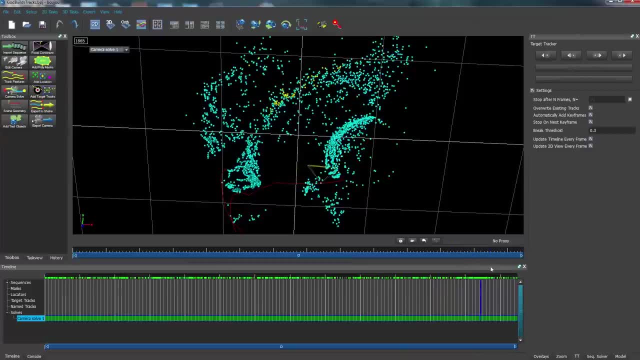 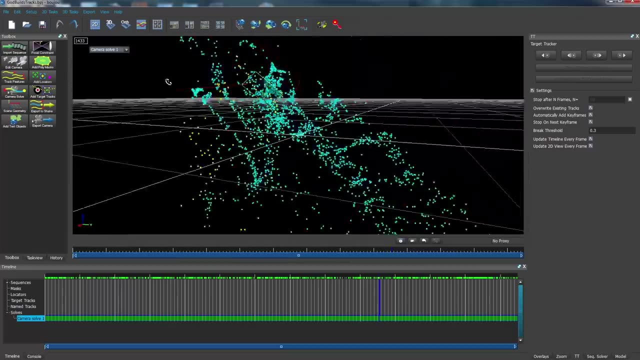 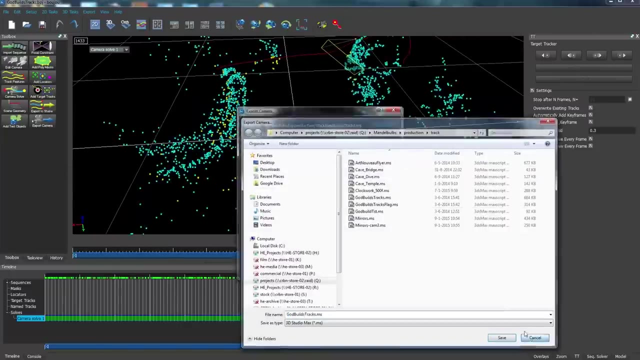 not very well with having a keyframe on each frame. so something like that hacking it- would be out of the question. also, you would have to adjust your rotation position scale of your camera path to something which makes sense in in the software Mandel bulb. in order to do that you might have to visualize the 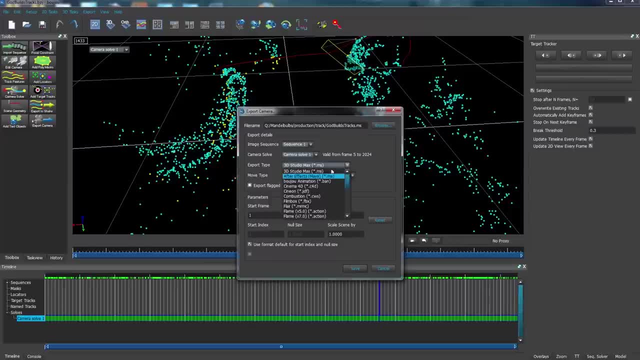 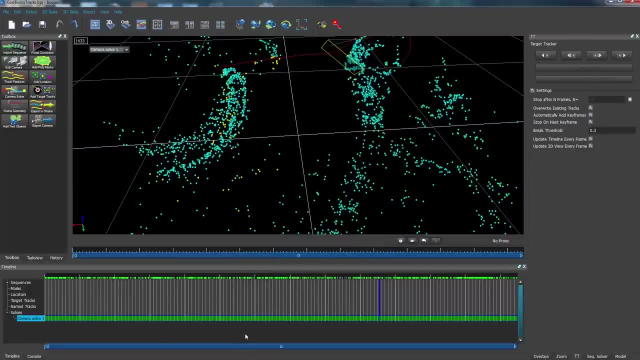 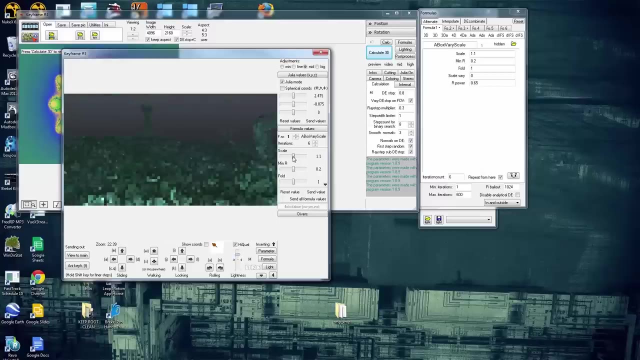 camera as a spline or something and then go to another view and rotate and scale. none of that is possible in Mandelbulb. so forget about importing camera data in Mandelbulb. but there is another, very you know it's not really a way to import it. 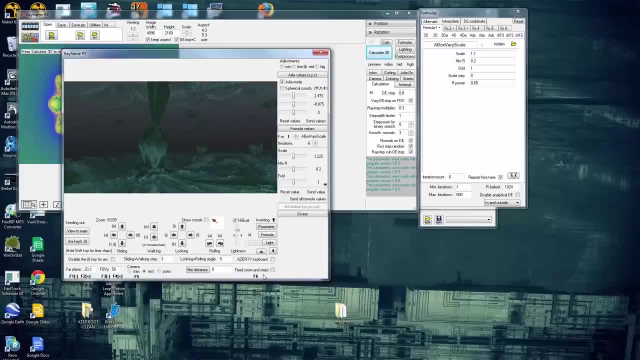 but it is in a way, and that is just by eyeballing it. if I have, if I maybe have an animatic or something with a camera motion, with a slight truck in and the lens is a 45 millimeter, then I can just look up what the field of view would. 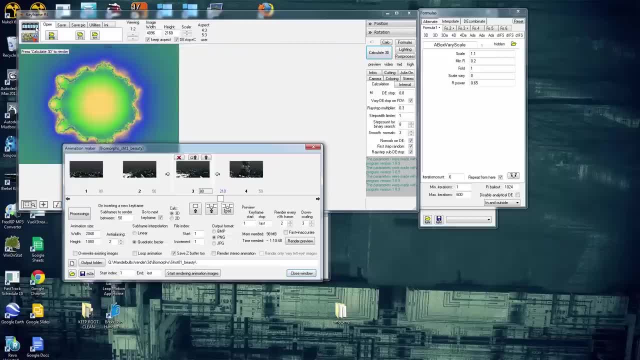 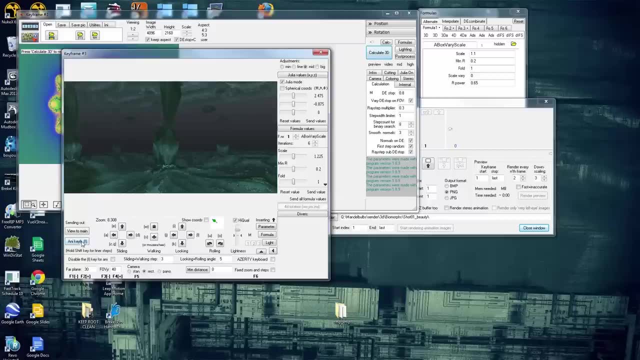 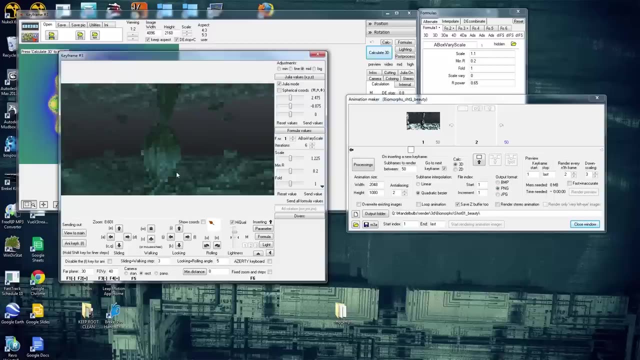 have to be. I can type in the field of view very exactly in Mandelbulb and I can do camera motion, which is a slight truck in over 72 frames or whatever it is, and like that I can recreate the camera motion that we would want to have. and then obviously nothing's gonna match if we 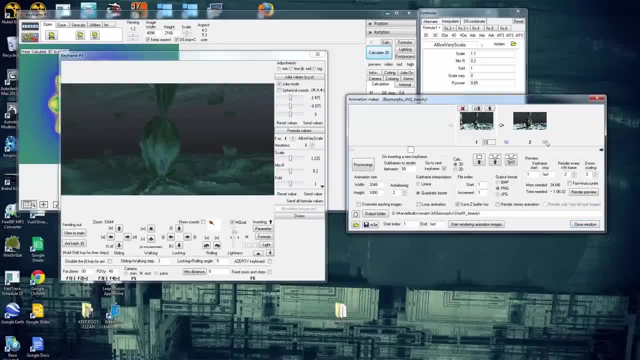 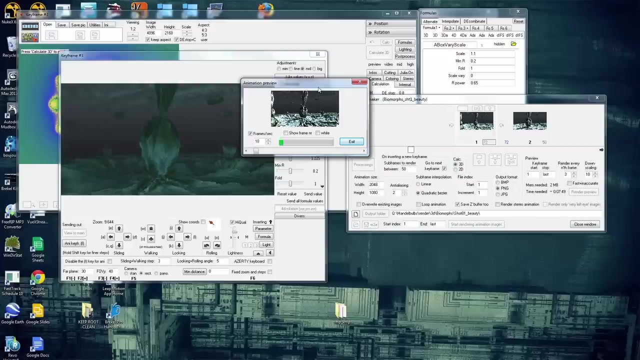 have if we filmed an actor or something. that's not gonna match. but then there are ways to actually then start tracking that camera from Mandelbulb, importing it in Nuke reprojecting and, you know, do whatever is necessary. but so the best result is basically had one when the camera motion originates in. 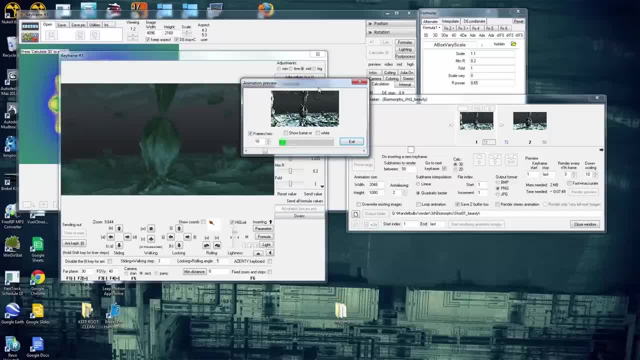 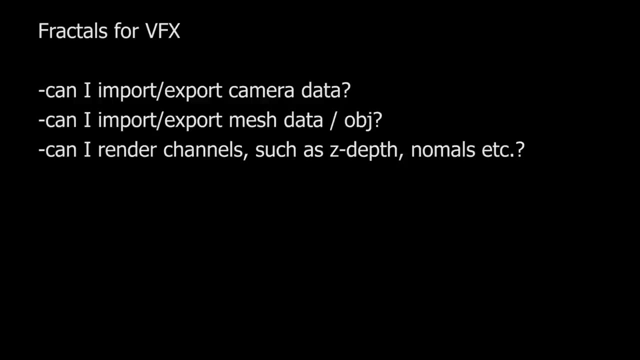 in in Mandelbulb and then it's exported, and which it's exported through the system of synth eyes PF track who's you works perfect. next question would be: can I import or export OBJ or and or mesh data? again, the short answer is no. unfortunately, again, there is no import, export or an OBJ. 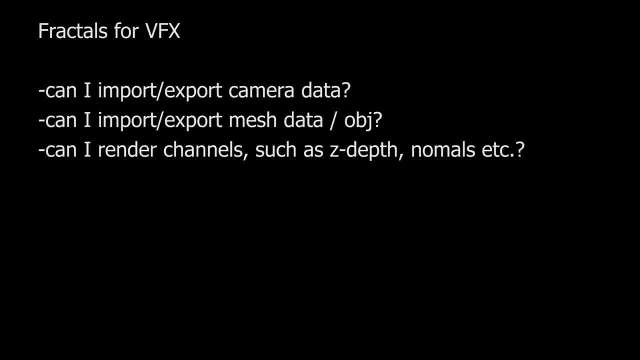 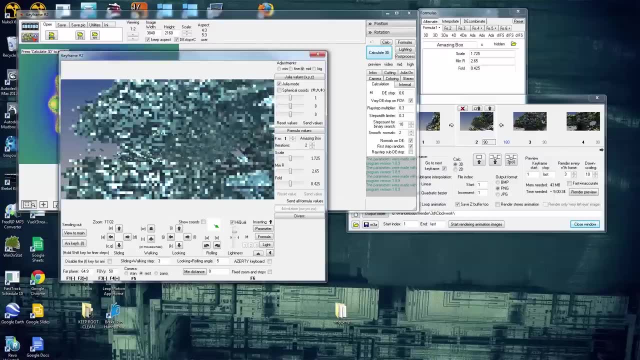 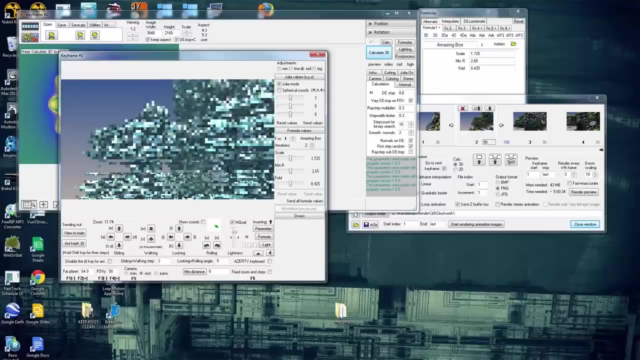 and if we think about it a little bit, then we can actually come to the conclusion that this makes perfect sense, because they aren't meshes, these rectangles. they are infinite, infinitely complex and obviously, at render time, there is a cutoff threshold and there's a. there is, there's a. there's a point. 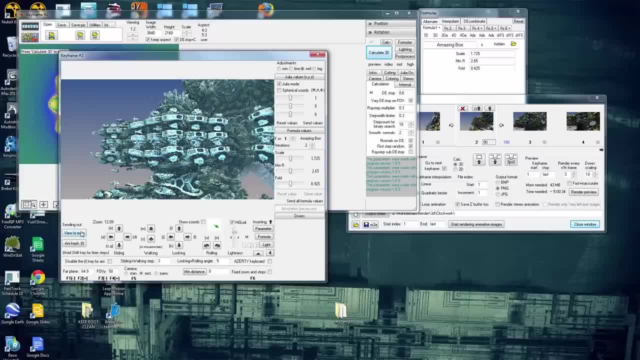 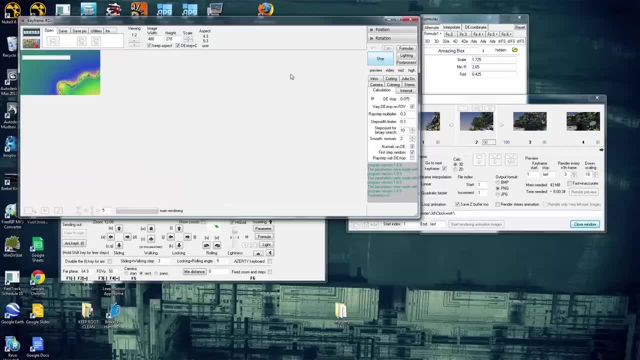 where, where it says OK, stop, stop iterating anymore. and I start rendering a dot on the screen. but this is going to it very hard to triangulate it and to export it. So the only way to export mesh data is something called voxel stacking. Basically, what you do is: 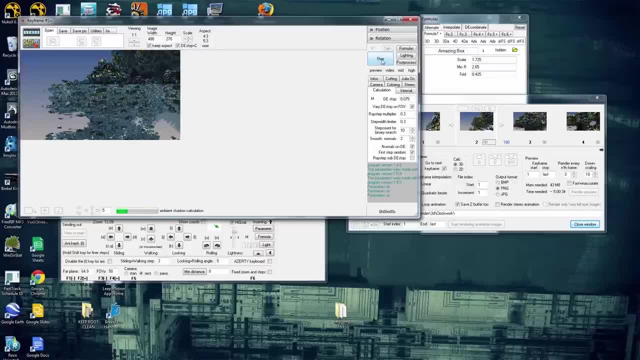 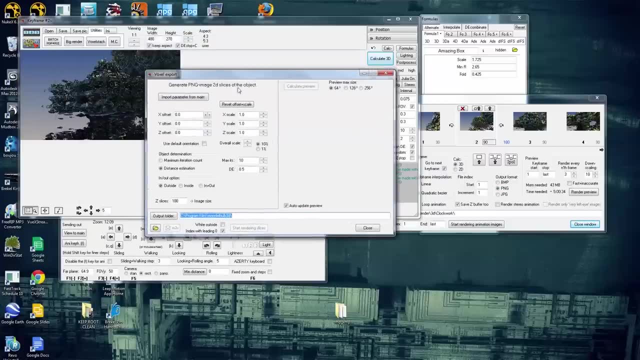 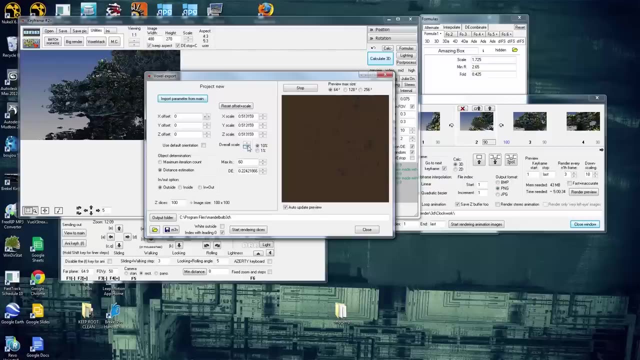 in 3D you define a voxel or a volume, which is usually just a cube, And then it starts rendering slices through that volume as PNGs or JPEGs. A little bit like an MRI scan would handle a three-dimensional volumetric, And what you get is you get a image sequence of black and white stuff. 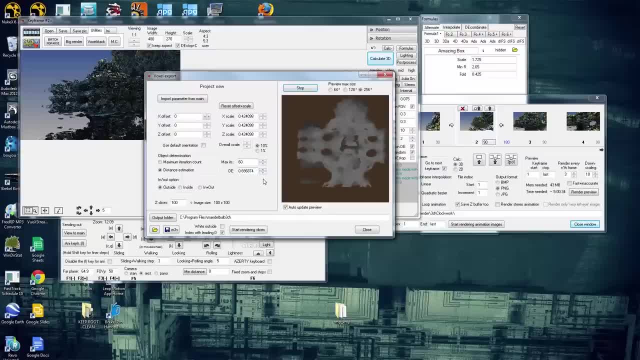 Black is basically where there is no empty space and white is where it would have detected fractal. And then it starts rendering the slices through that volume as pngs or jpegs. And then it starts rendering the slices through that volume as pngs or jpegs. 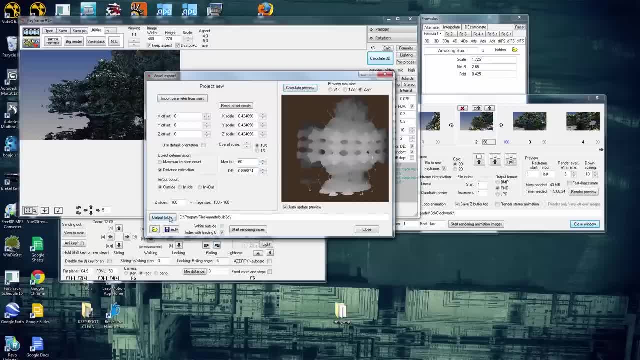 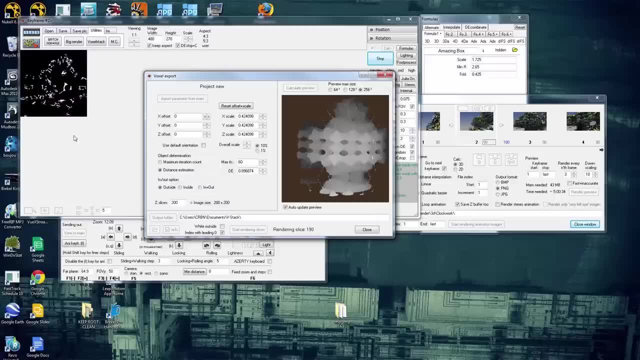 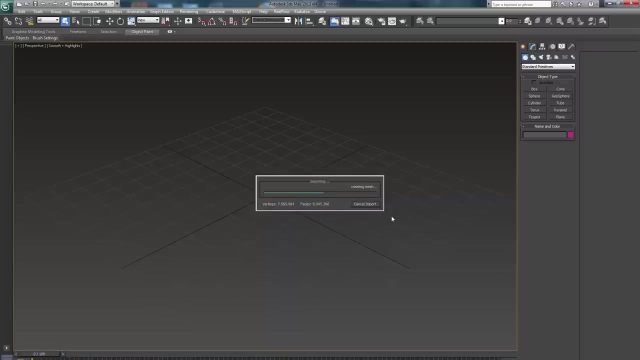 I can take that voxel stack and I can run it through something called this is VJ Fiji, this is Fiji, or J Fiji or something like that, and that will compile it into a OBJ. so in that way you can actually export a piece of your fractal. be advised, it's only a very small portion of the fractal and it can. 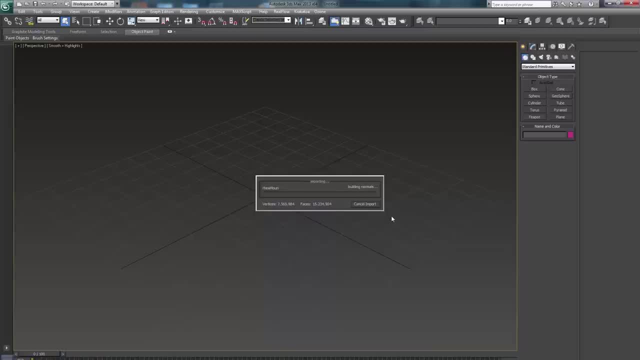 export it into it into an OBJ, and that OBJ will be very, very, very, very big. be like if it's a thousand by a thousand by a thousand voxels, I think it can be well over a gigabyte and it can take very long time to compile it in that Fiji. 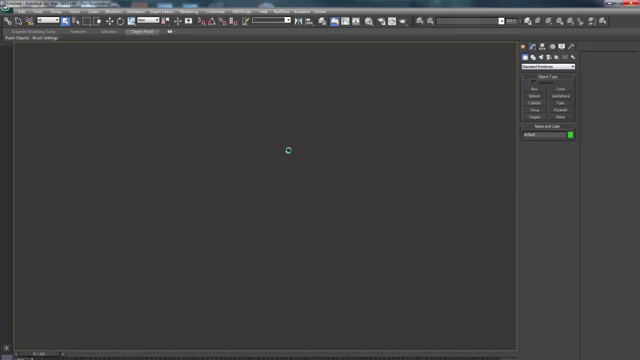 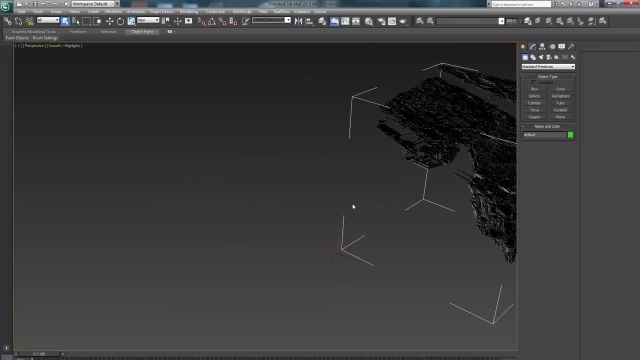 program and then you need a lot of cleanup. you need to go into ZBrush and you need to. you have a lot of extra layers as well, because you need to have a lot of extra layers as well, because you need to have some fractals. they're like an onion, so you only see the outside, but actually 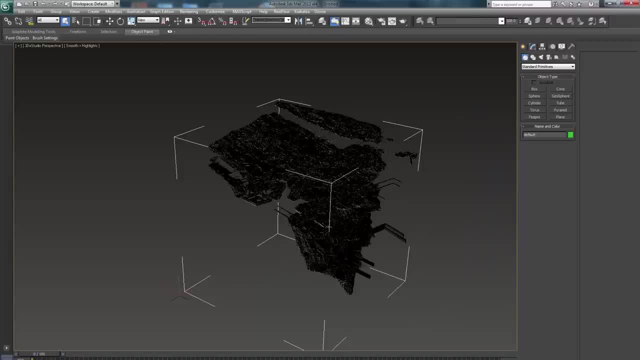 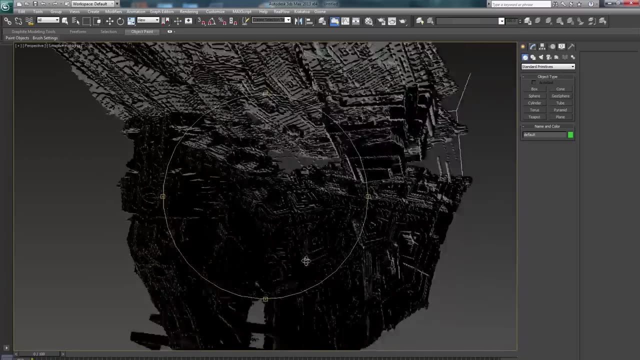 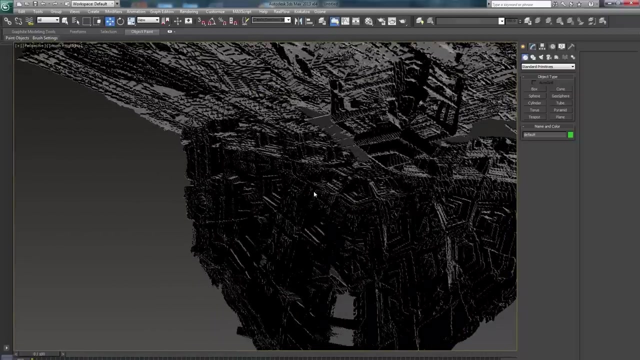 inside isn't just solid, it's lots of tiny layers and and obviously the software has no way of knowing that you're only interested in the outer layer, so it will also take all those inside layers, and this can be very, very high-res. so this is not at all an option that I recommend, unless for very 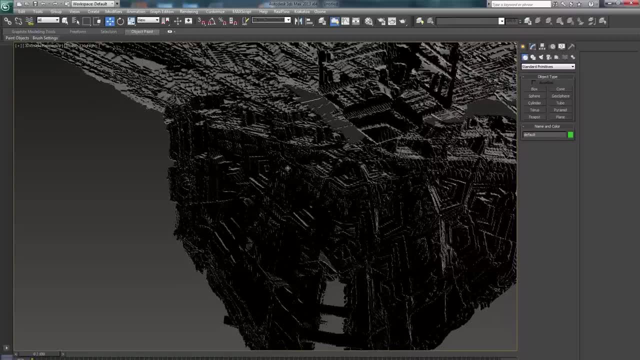 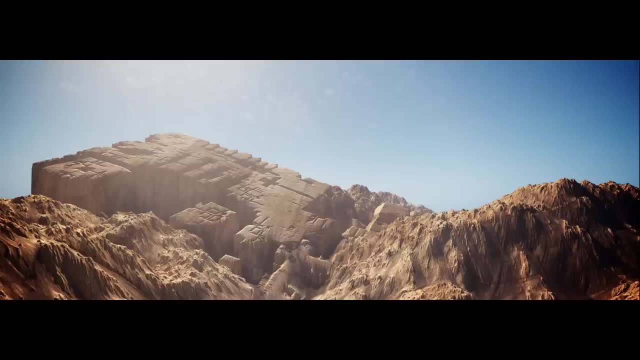 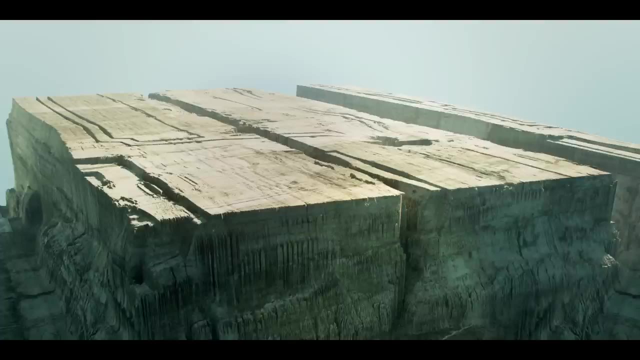 specific stuff. another way of of doing it is looking at it more like a, like a hide field terrain. so I actually, if you are, if you're looking at a fractal more like a, like a, like a mountain scape, for instance, and again, be advised, these are 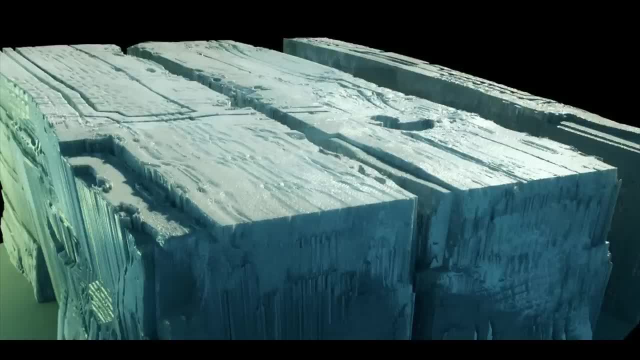 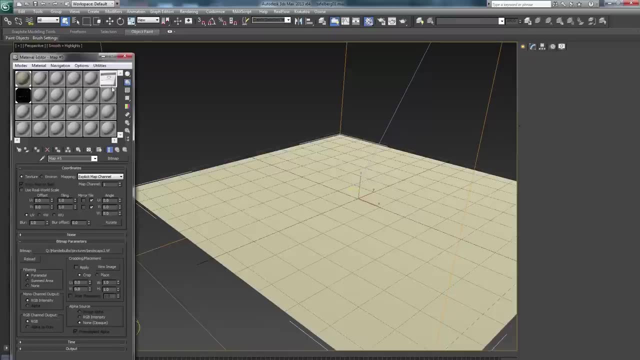 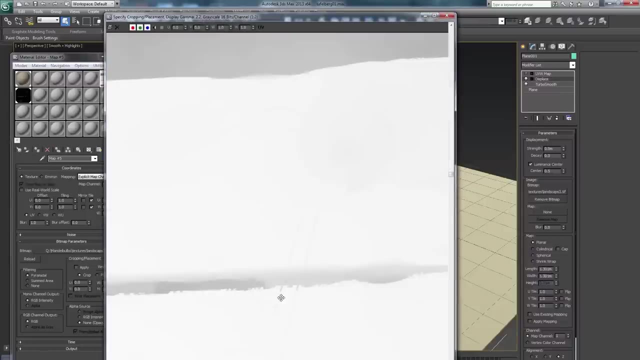 not fractals that, like you find them in in vu or terra gen or something they're also called fractal, usually making these mountain scapes. but they're like you're Questono exactly how it works, but they're like random noise functions with fractal properties. but they are not the same as these type of fractals, as these: 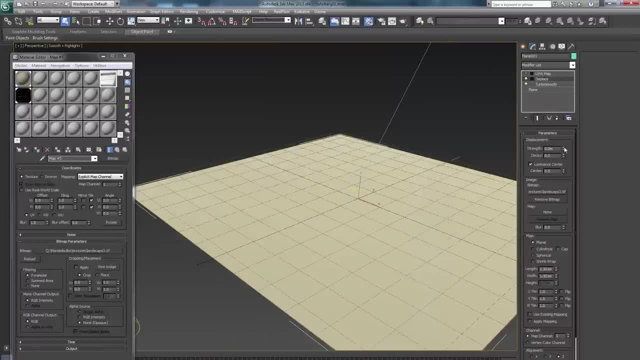 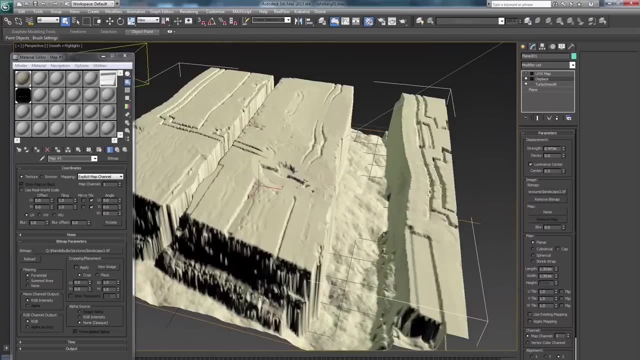 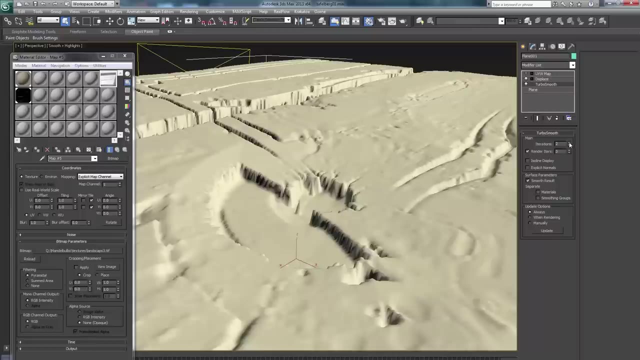 proper fractals. so for these proper fractals, what you could do is you could from top down. if you have a something is that resembles a landscape, and it can happen- it can't have any overhang, as it is, as is always the case with with hide field terrains. you could from top down drop. you could from top down you. 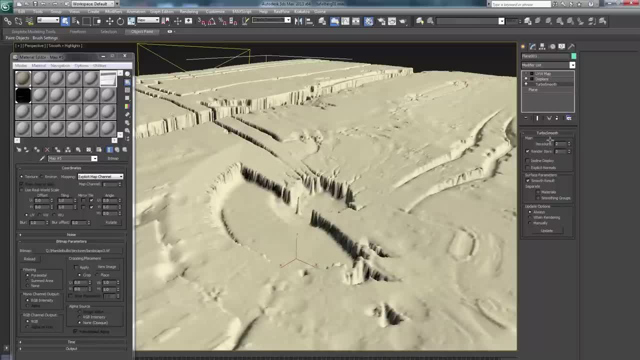 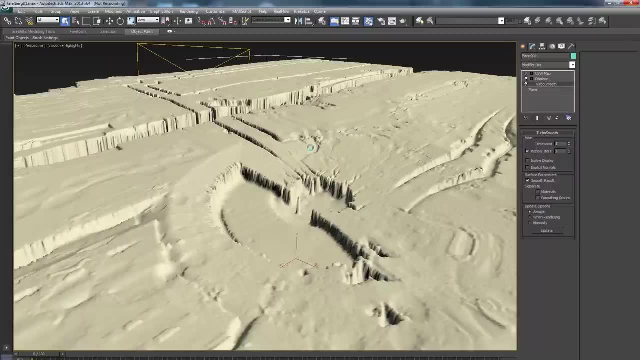 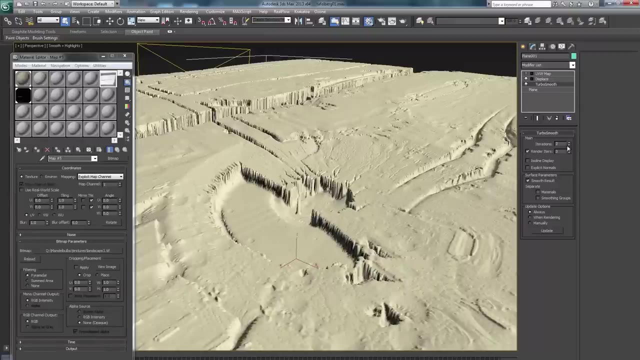 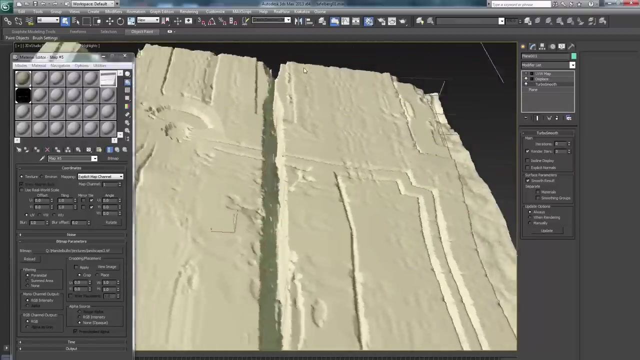 you could voxel slice the terrain and you could do that really high res. it can be like 4k by 4k, by 4k, because it's a volume, volume. and then take that. and then a colleague of mine who works at hectic electric called julik tarkanov. he wrote a nuke script that does exactly this. it takes 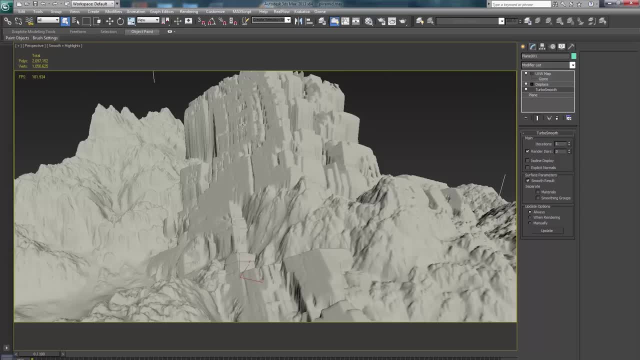 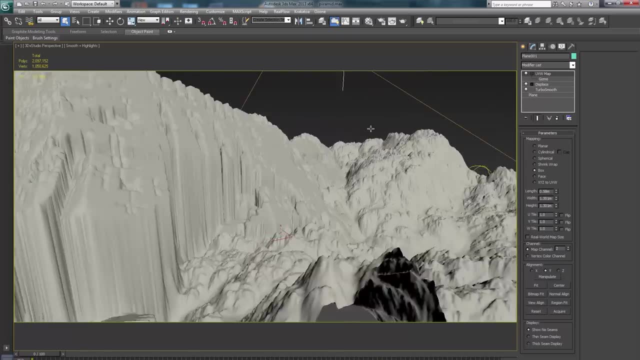 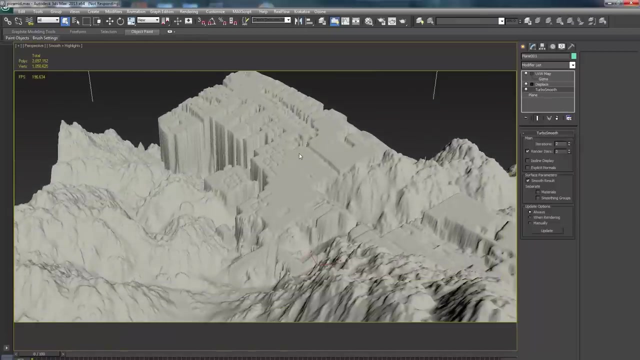 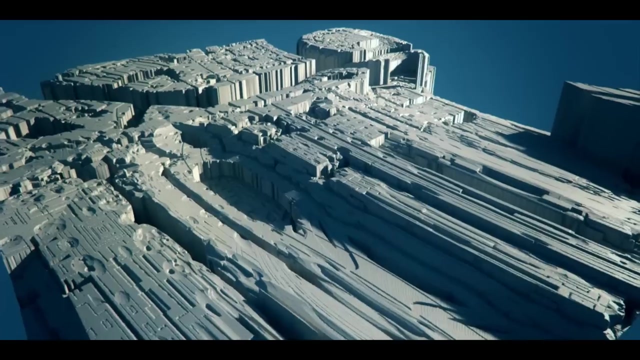 these voxels and it stacks them on top of each other and it creates a 32-bit exr height field terrain, which is basically only one 4k by 4k bitmap. and if you, if you then take that into maya or or 3ds max as a displacement, you really have a lot of detail, but you can't have any. 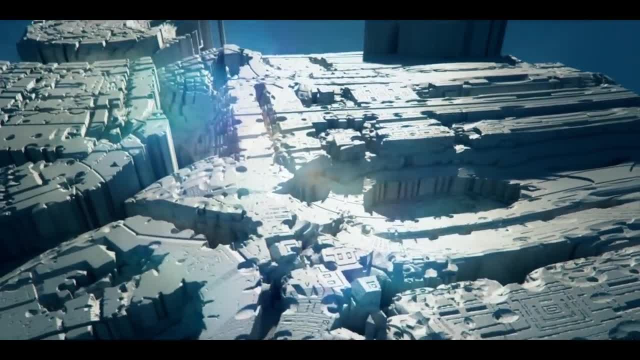 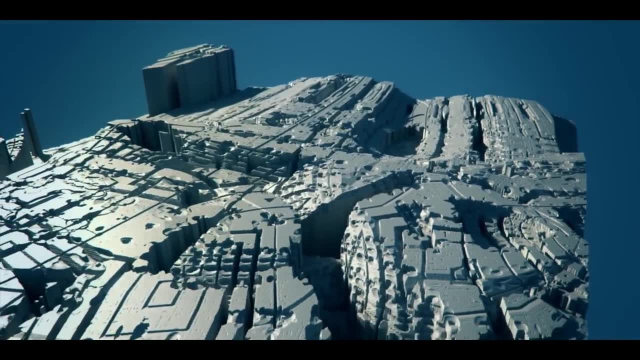 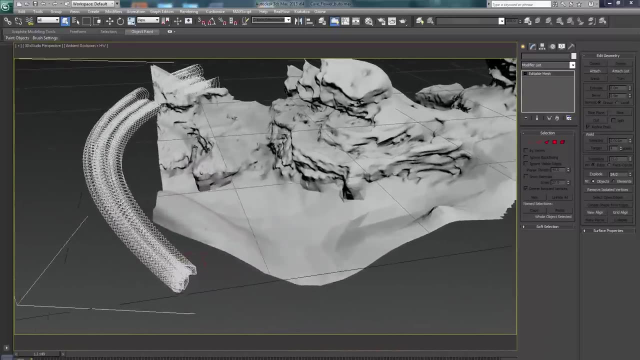 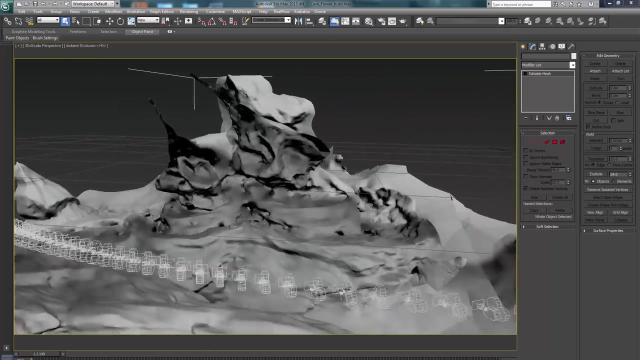 overhang but it's great for for um making a fractal to range. so this is another way of exporting mesh data. there's one other way and that is similar to exporting camera data. as i said before, if we look at a nice part of the fractal that we like and we we render it with a moving camera we have. 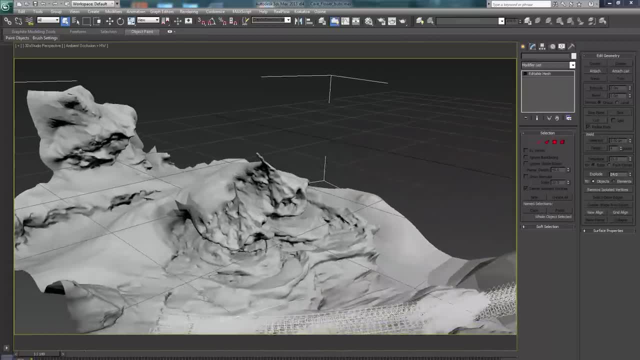 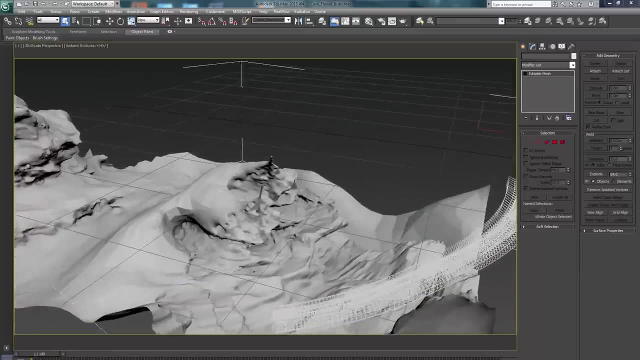 some parallax. we have a lot of parallax. we can easily render like 100 frames or something that we rotate around it for, uh, let's say, 90 degrees. we render that and then we take those stills and we we feed them into software called. 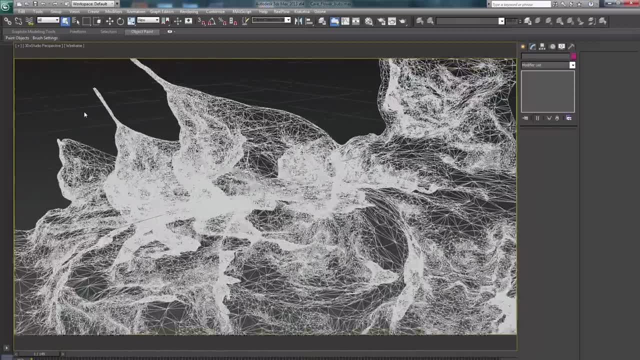 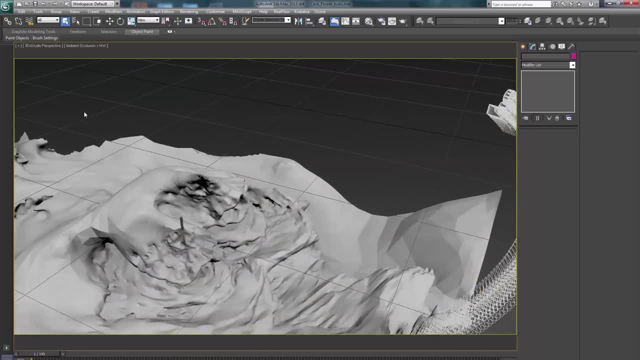 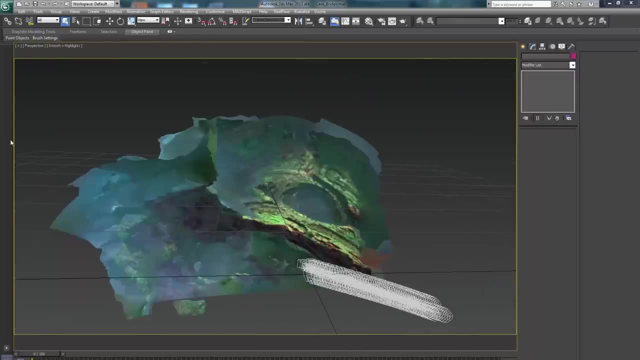 photoscan by agisoft. so photoscan will- um, well then, first it will. i think how it works it's it's actually the same stuff, but it works much better than a one to three d catch by autodesk. uh, it will actually first like track the camera a little bit or find similarities and it will build a mesh from. 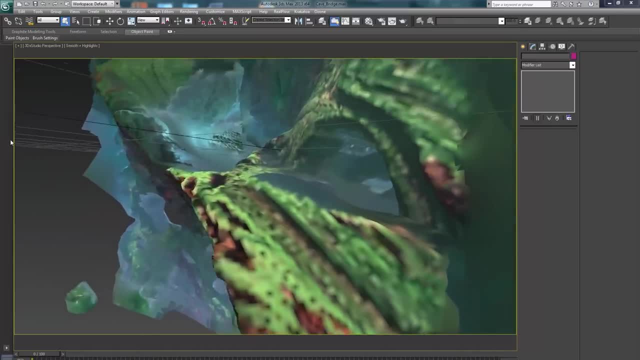 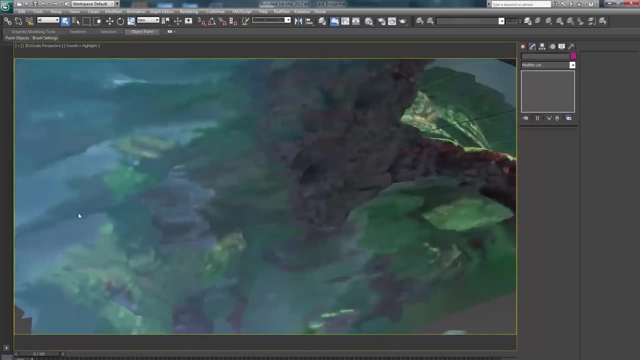 those different views. it's actually more it's made for for photos, so you can actually also photograph your house or a mountain or anything from different angles and it will make a mesh, constructed mesh, from that. it will do the same thing with a fractal and this will get a. 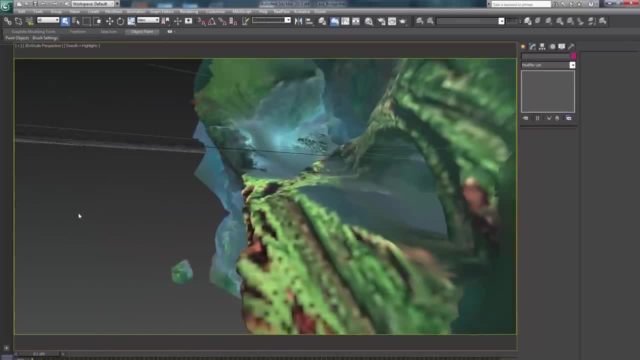 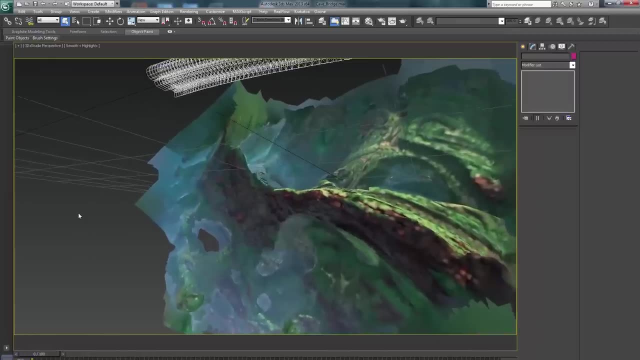 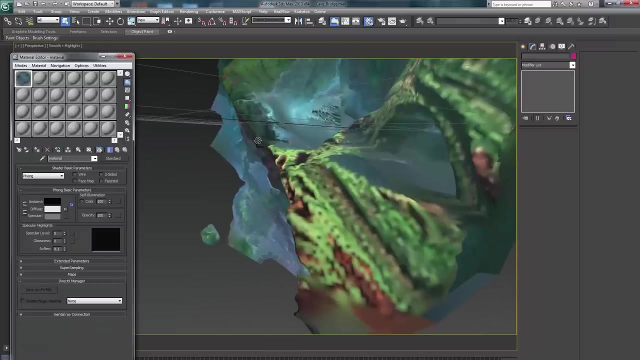 very high, high res mesh which is great for then putting other stuff on and using in your pipeline, but it's not high res enough that you can relight it and completely get rid of the texture, and you will still. it will still look like the typical um uh photo scan. 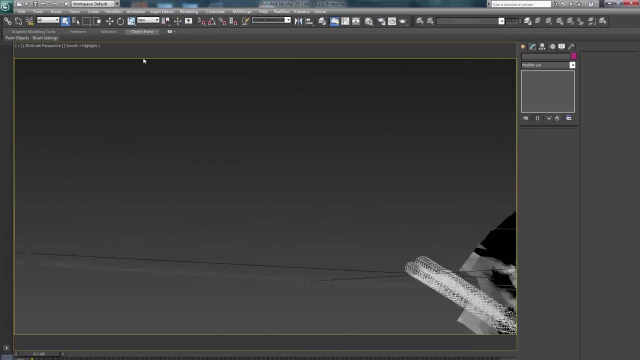 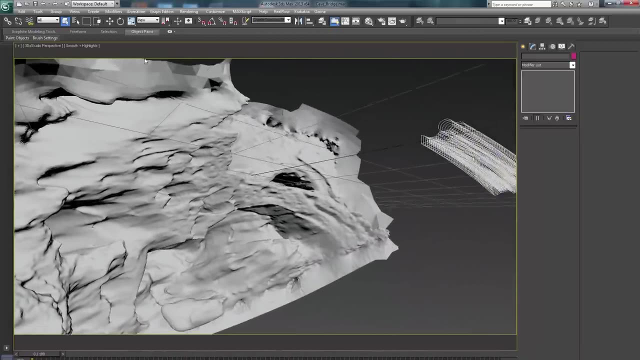 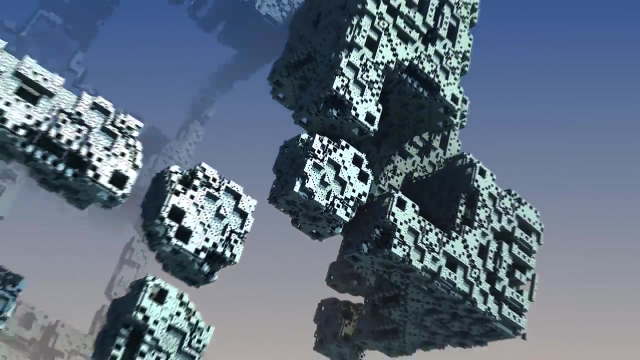 and one-to-three the cache, one-to-three the catch mesh, but very high resolution. so this is another way to export it. um, importing is not, is not possible at all. uh, i did have the suggestion from someone. how cool. or someone said to me how cool it would be. 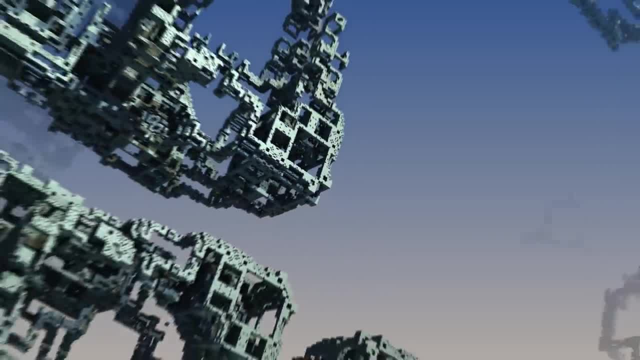 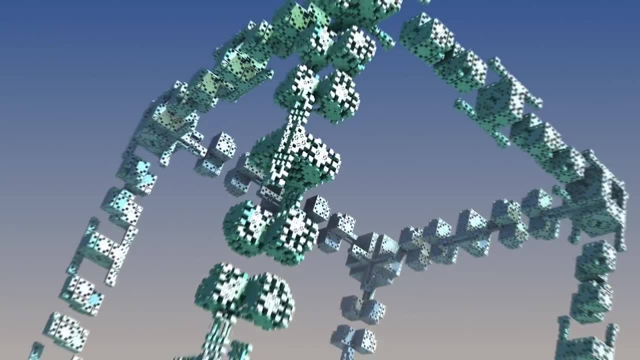 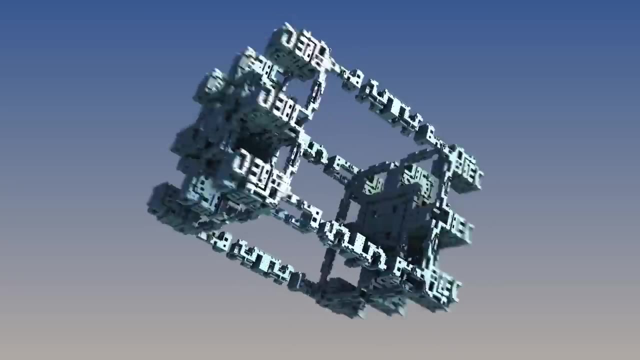 if you could import an obj and then grow fractals on on that structure, so you could. So if you could import like a really rough layout of a terrain, maybe, or of a building with walls and ceilings and not much else, and then it could just grow fractals on that, that would be totally awesome. 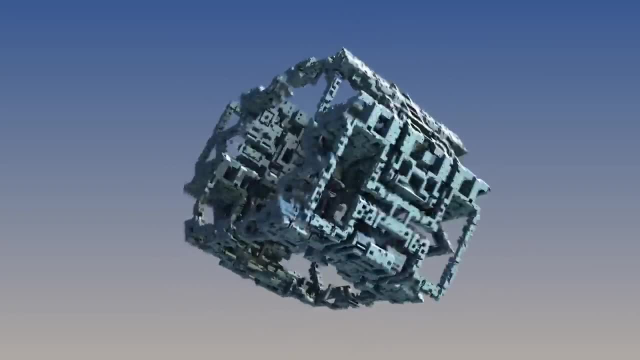 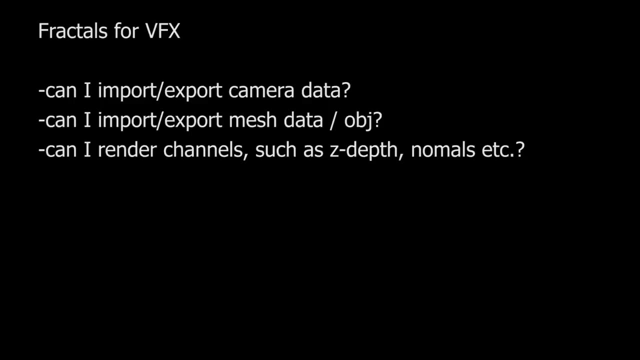 That would be really amazing if that was the case. Unfortunately, nothing near that is possible. So another question I often get is: can I render elements or channels like normals- reflections, Z-buffer, et cetera? You can render a Z-buffer. 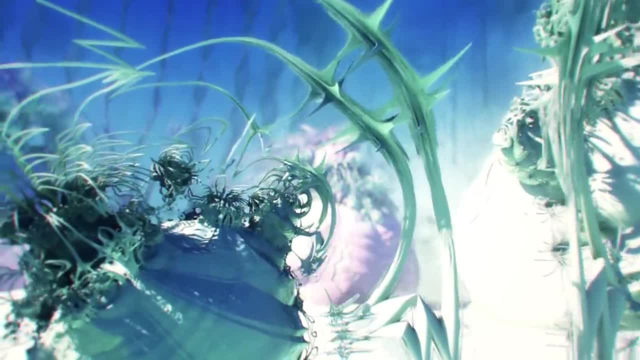 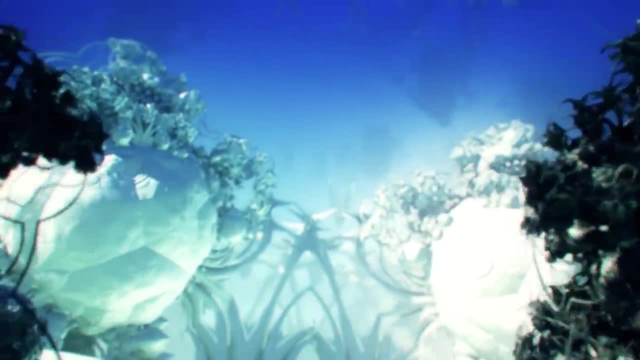 It's actually I do it all the time. It works just like another software. The only thing is it's only 8-bit, but it could still be very good for stuff like in compositing. You can do clipping, You can do like fog in the distance. 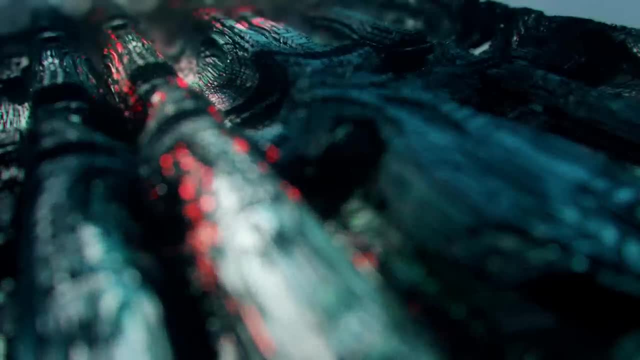 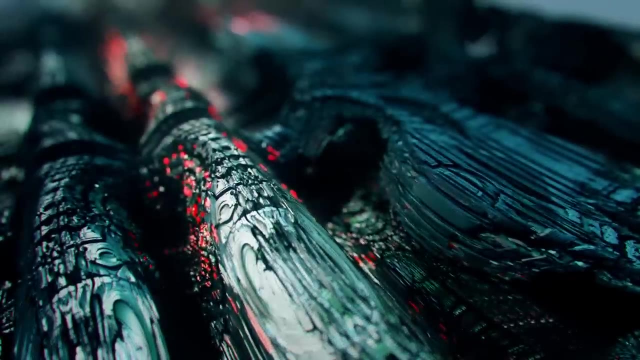 And you can do depth of field, which works great also with 8-bit, so that's really perfect. I use Frischluft and you can do some great depth of field stuff, So there are lots of good ways to use the Z-buffer. 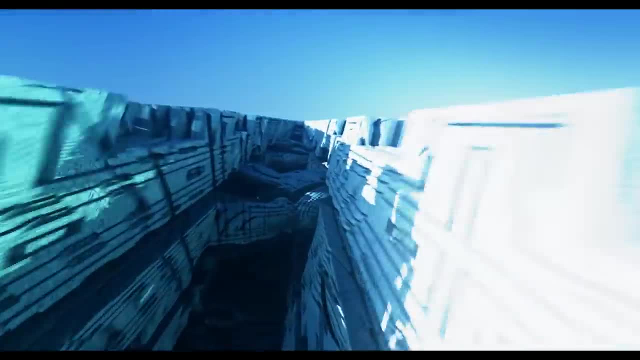 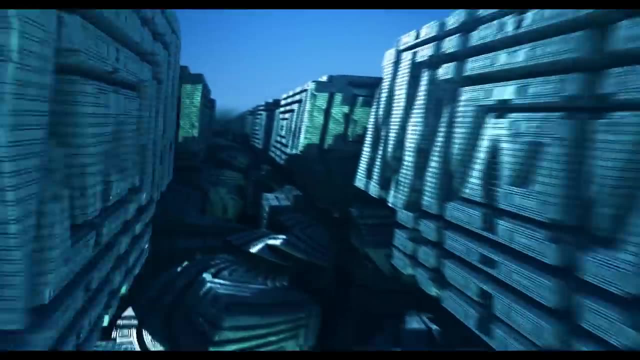 That's really one of the things that I started like looking more seriously at Mandelbulb when I found out that it would do that. It's like, okay, I can really. I can actually use this, I can actually go in now. 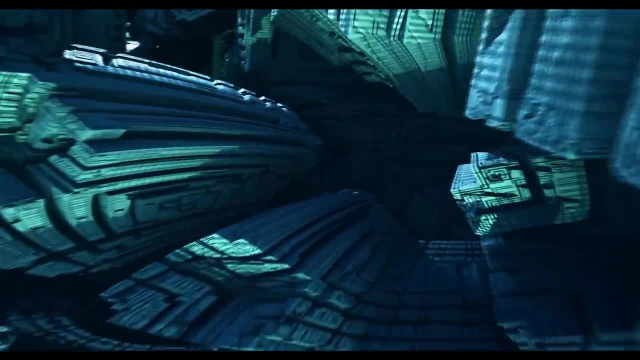 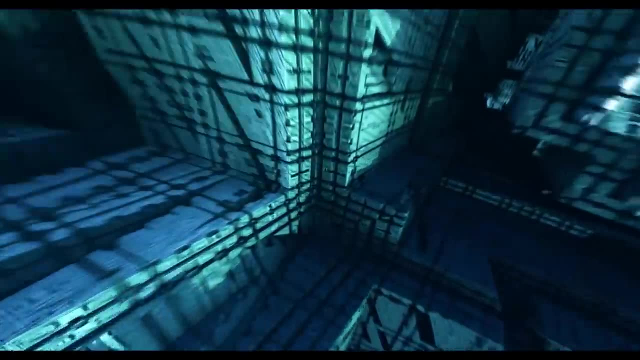 And start compositing with this because of that Z-buffer. So that's a very helpful one and that's the only yes you'll get, because the other things- normals no, reflections no- But again, there are ways to get normals and reflections because it has reflections. 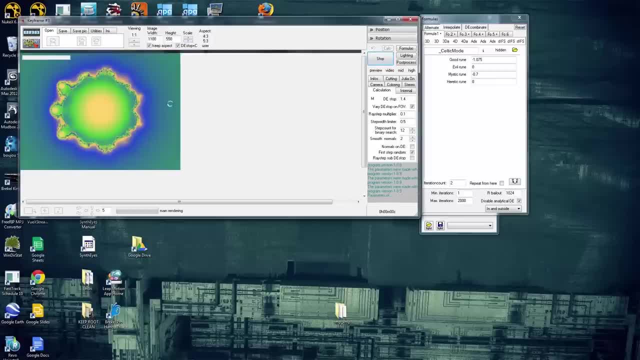 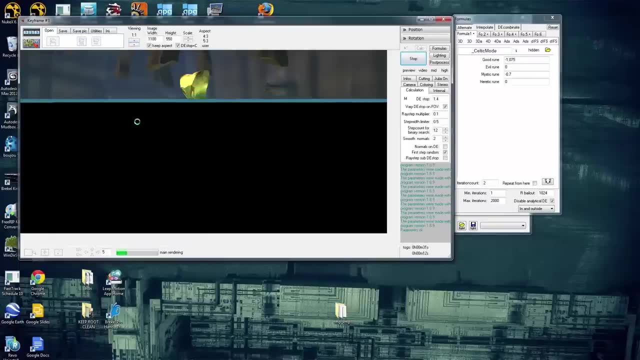 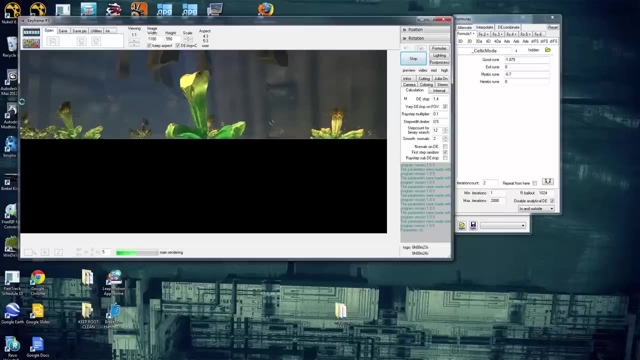 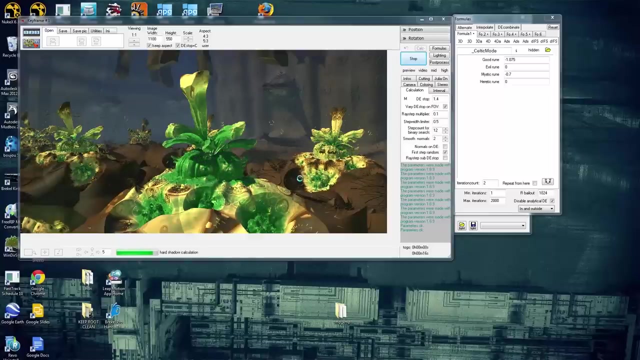 It just won't have a separate channel for reflections. But if you render one pass with reflections, you're just a beauty render and you render the same render after that, again without reflections. So you are rendering double, so which is a lot of waste, but it's then. I could in my compositing software. I could do a difference between those two passes and I would get just a reflections pass. 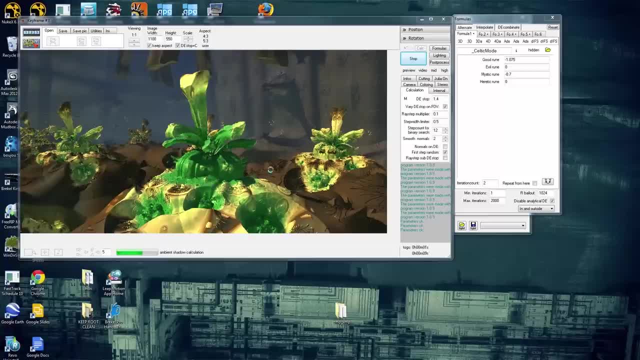 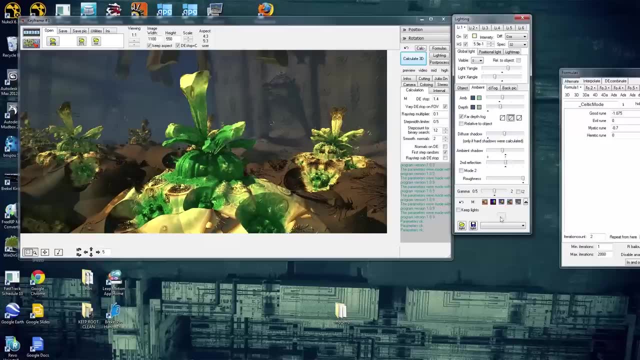 So in that way you could get a reflections channel And same with normals. There is actually- Mandelbulb has a way of it does know the normal inside the frame buffer. There's just no way to export it, But you can. 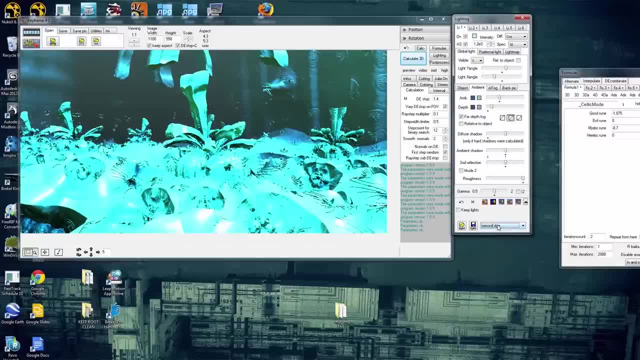 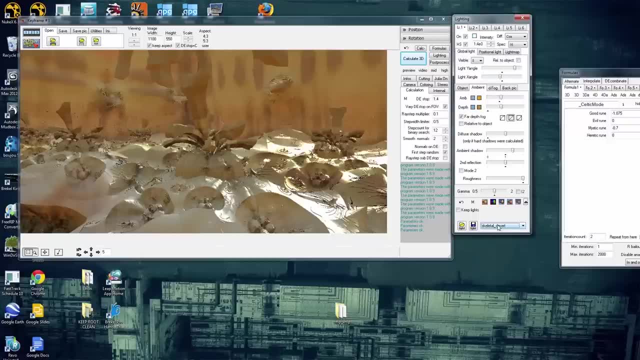 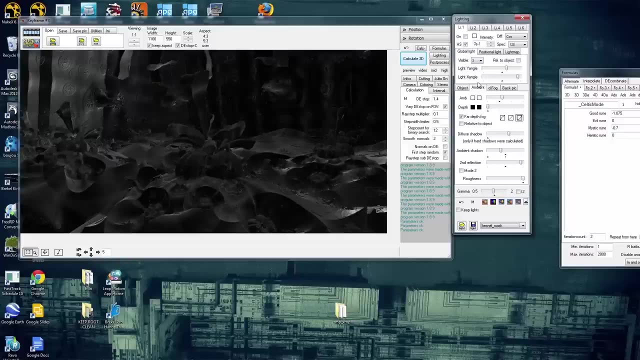 You could take a bitmap and have it look at the normals. have the UVs of the bitmap conform to the normals or something like that. I haven't completely explored it, but I can imagine if you take a bitmap which is just a red, blue, green, yellow for color gradient, or something like that. 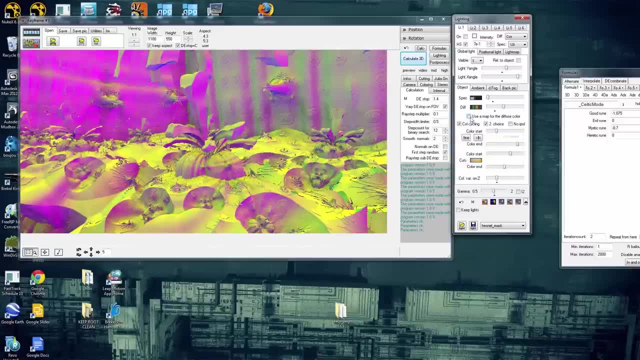 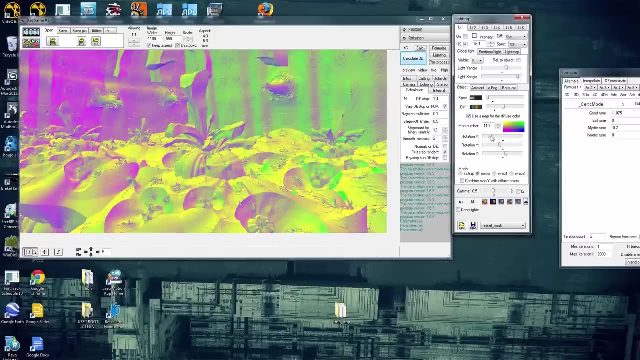 you would have to work out exactly what it is you'd need to do, but I'm sure you could figure it out And you feed that in as a bitmap, While killing all the ambient occlusion and all the lighting and all the shadows, et cetera, and like having it as a self-illuminated material, as it would be called in Max. 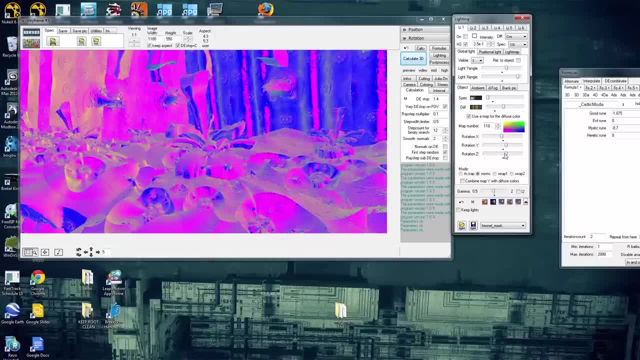 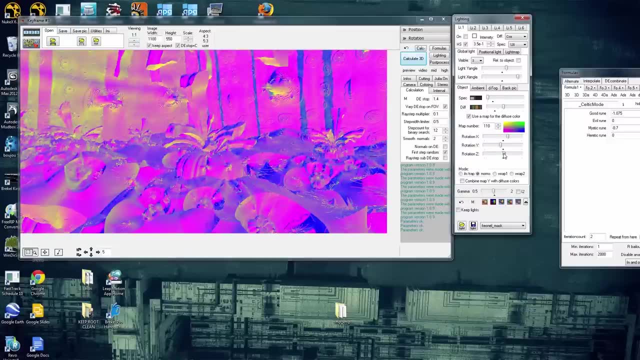 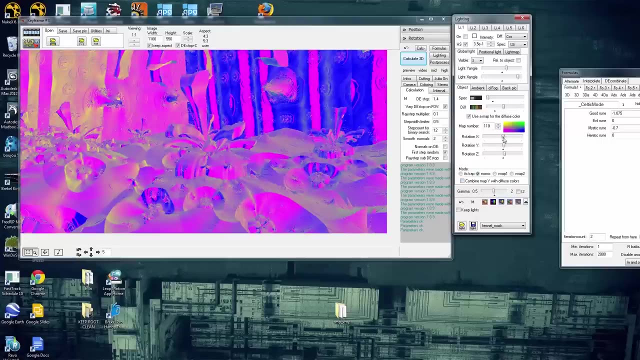 and you'd have it conform to the normals, then you should get a usable normal pass. but I think it's difficult to set up and it's not usually not really necessary to have a normals pass, but I can imagine That could be used for that. 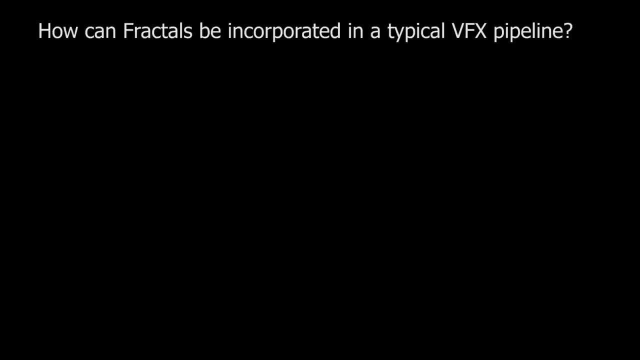 So how can fractals be incorporated in a pipeline? I've gone through, I've gone over a couple of things, but I've also said there's a lot of restrictions here. It's going to be hard to say. you know, you come into a studio and just go. okay, can we use this? can we make the mountain scape for this alien landscape on it? 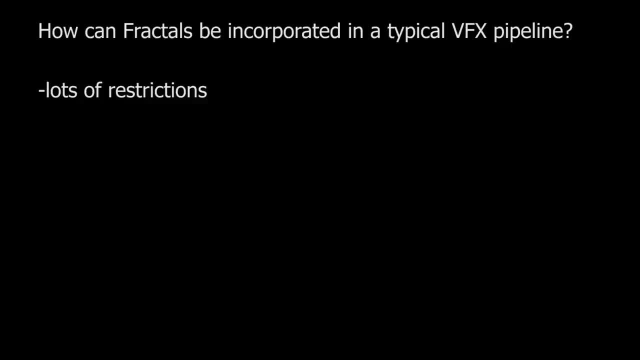 And I say: well, here's a good idea. we can't import the camera. we can't export the camera, we can't really get some geometry to to match with it. so there's going to be a lot of problems that we have to overcome, indeed, there. 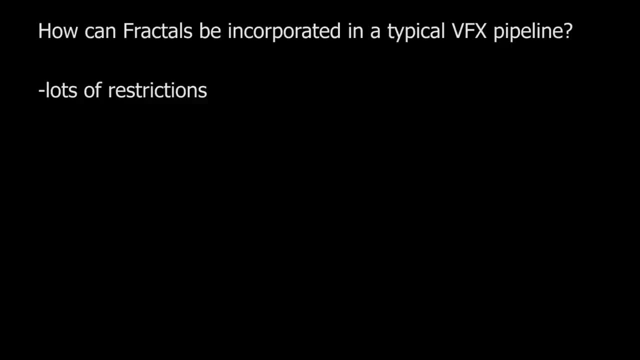 are and some part of the solution could be. i'm not saying it necessarily will be, because it depends on a lot of other factors, but it could be that you change your pipeline a little bit. you just say, okay, we, we love this, these fractals, we love this. look, we want to go with that, but we 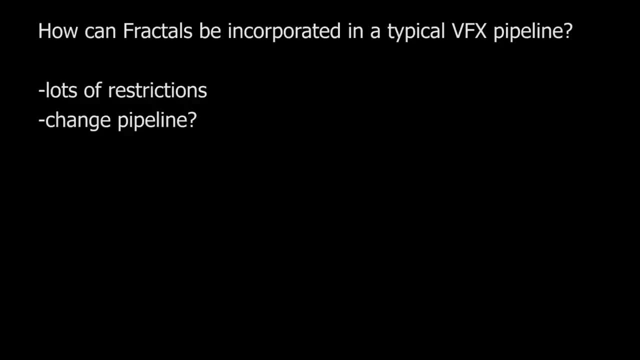 have to, um, to start a little, just just to change a little bit the way uh, we we think about how this stuff usually goes, because usually you know, if concept art or, and then it's good, maybe goes to them to do to the matte painters or, and everything works together and maybe with this kind of stuff, 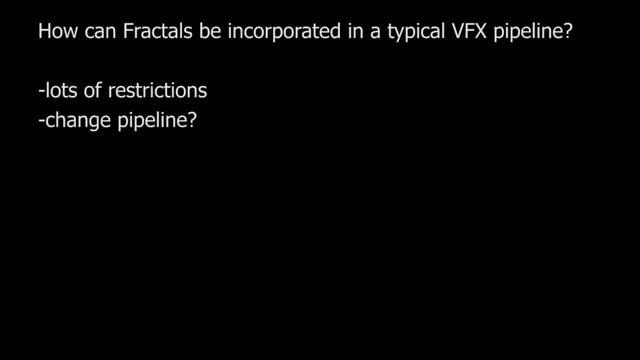 you would have to change that a little bit. which is not the end of the world. and, uh, i'd like to, to, to maybe give one idea of looking at it, just one um way of seeing that that it maybe it hurts less or it can be more fun to do it. and this is, uh, which i call fractal recce or fractal location scouting. 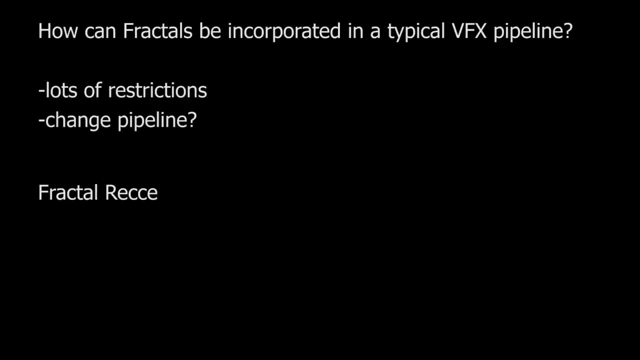 uh one, when we are writing a script for film and then at one point some location scout is going to look for the locations and he's never going to find exactly what's in the script. he's all he's. he will probably find completely new things, or he's going. 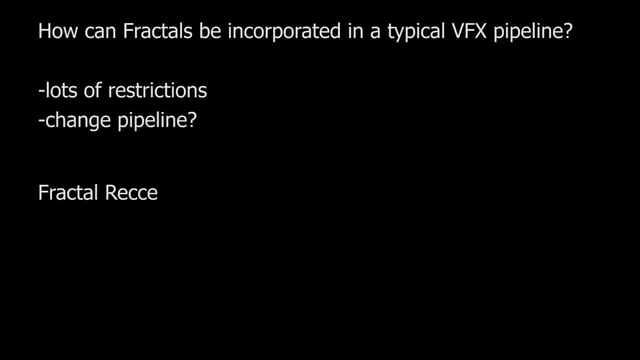 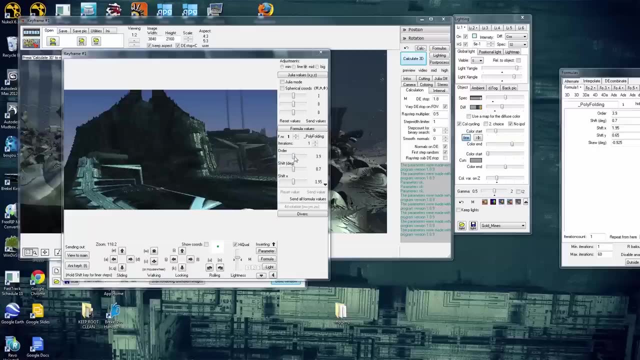 to say, oh, hey, this location would be great. and then the producer or the director might say, well, that location looks great, but it doesn't work for this scene. but hey, it could work for this scene. so these kind of things, they change all the time and a location obviously. 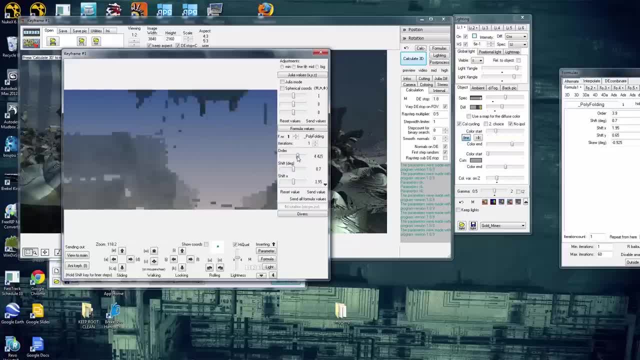 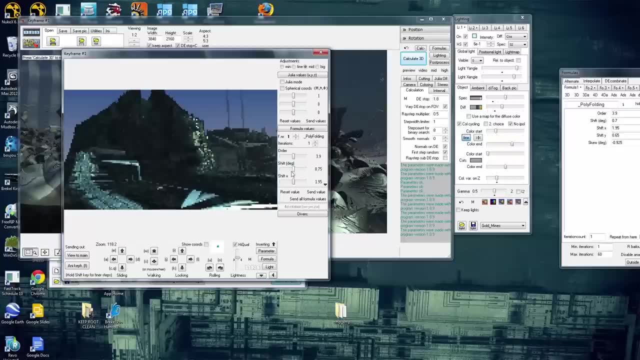 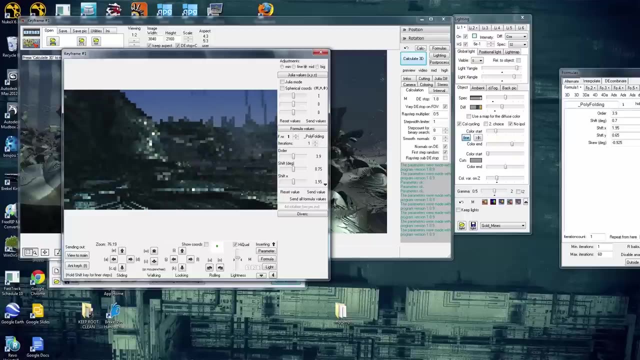 will never be known at the moment the script is written. so the location is a big variable and it's often you can't really change much about a location, or at least this is how it used to be for the last 50 or 100 years. obviously, now we are changing in visual effects, which we're changing. 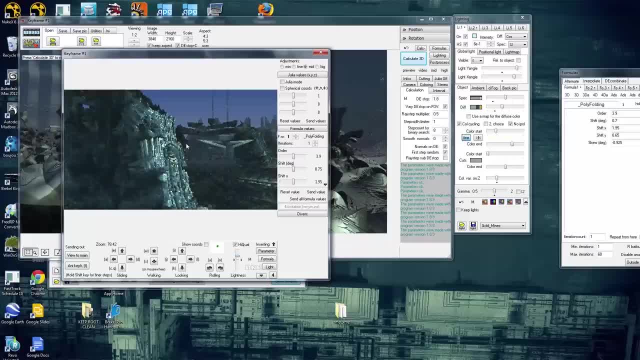 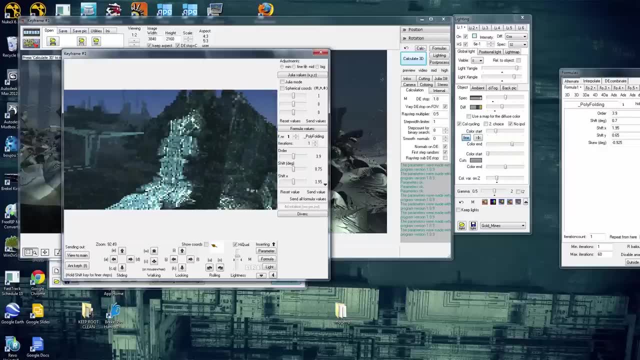 a lot about the location, but imagine that we weren't. then we'd be at a location and we'd be, let's say, at a mountain. we used mountains before we have a mountain, we have a lake, and then we start looking. well, where can we put the camera? 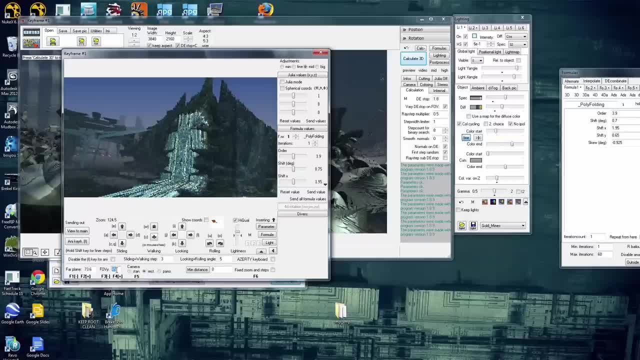 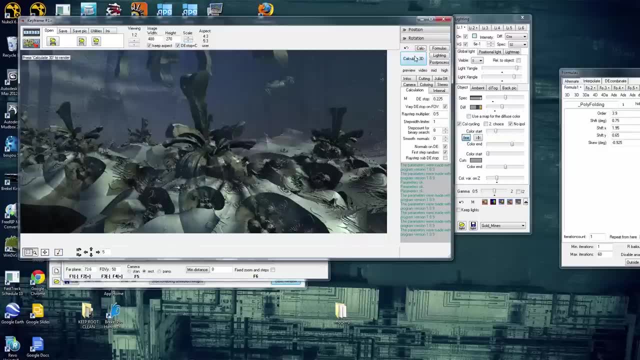 which angle can we look? where's the sun? you know, everybody's cool with the fact that we can't change the location of the sun, that we can't change the shape of the mountain, we can't change where the lake is, but we can change where the camera is and which way we're looking. 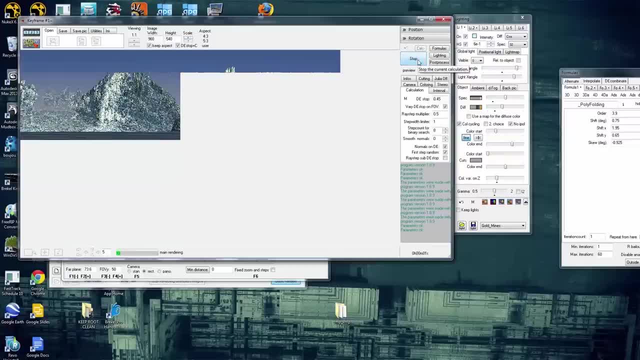 so this, this is what, obviously, cinematographers do all the time they're in a location, and they need to. with what they have, they need to make the best possible picture. well, imagine doing the same thing with fractals. imagine that, even though we have all this power to change the fractal, 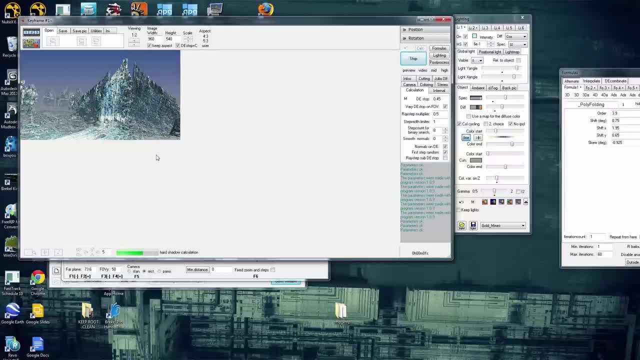 we don't have some power, we we cannot exactly define: uh, can we close this more and but keep this shape over here. i like the shape over here, but we need something here. we can't always necessarily do this, but we can completely. we're completely free. and where we put the camera? 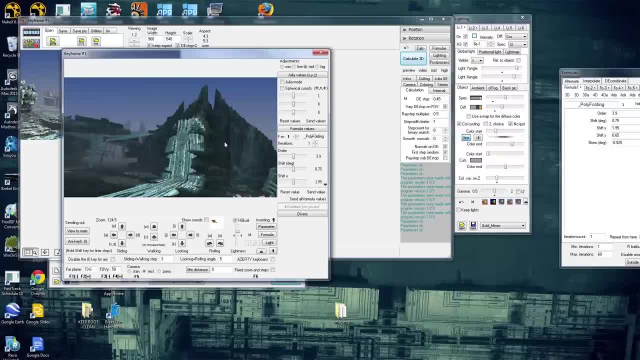 also where we put the sun, in this case. so we have more freedom in a way than a traditional location scout has. so, fractal location scout, we go inside the fractal with. uh well, we go inside the right fractal, we, we want to have a this particular kind of place. 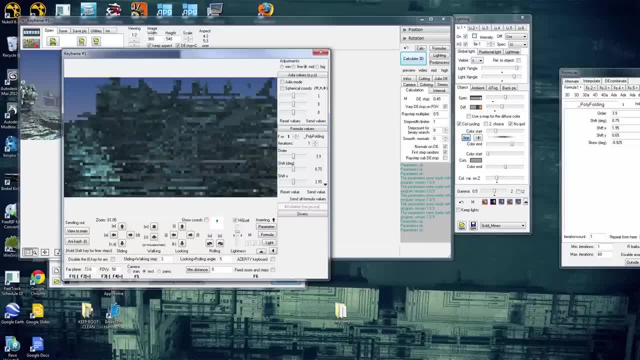 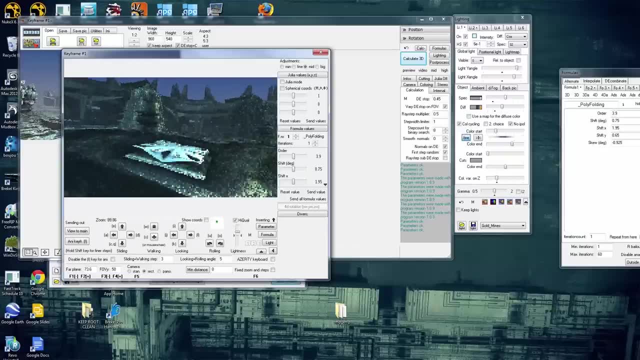 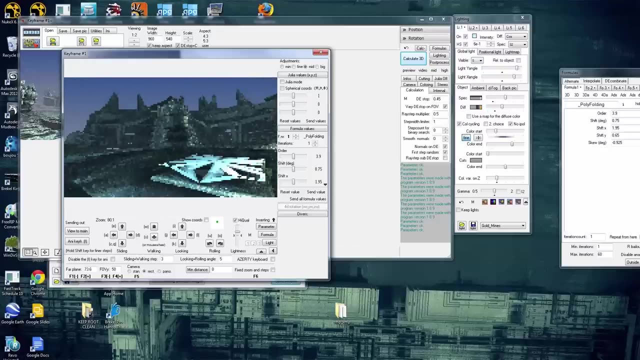 so with that mindset we go in the right- okay, this kind of thing. and then we start looking until we have a beautiful shot we think that could work for our film, or maybe not a shot but a motion that we can work with, and then we can actually, inside mandel bulb we can render these bits. 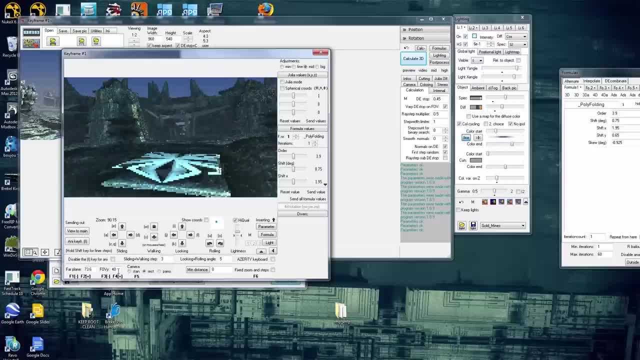 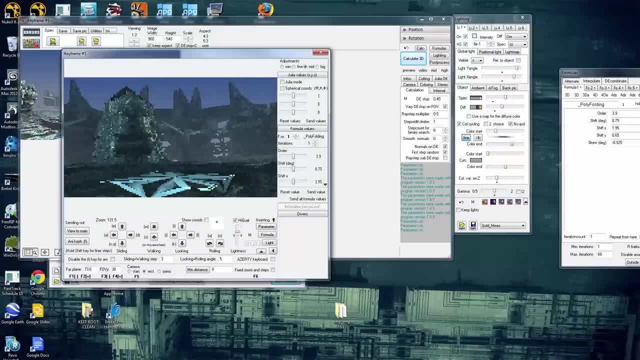 we can take that bit and voxel, slice it, do something else with it. so thinking about fractals in that way can, i think, immensely help. and this can help creativity, because you're obviously you can be very creative on a very narrow scale. there's a lot of stuff you can't do, but because there's a lot of stuff you can do, you 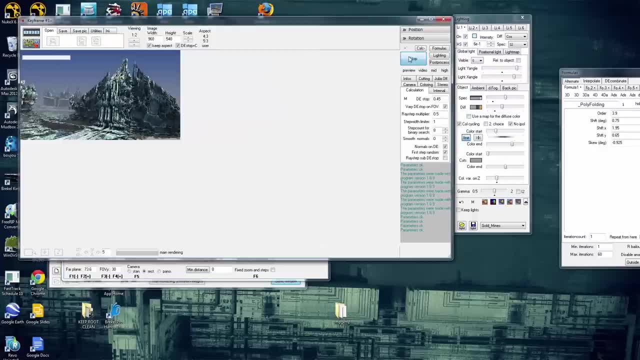 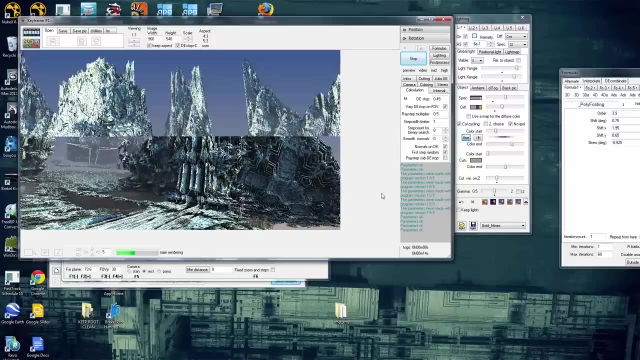 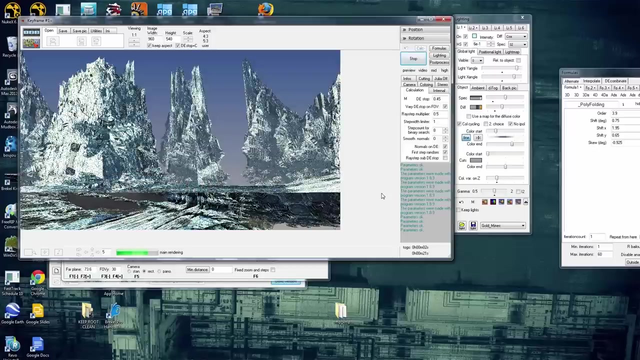 have to be very creative with the stuff that you can do- and it's actually surprising how much stuff you can do, uh, using these fractals- and i just think that, um, this, there must be some really cool cg short or film or maybe title sequence or something like really big and uh, not necessarily high budget, but high profile. 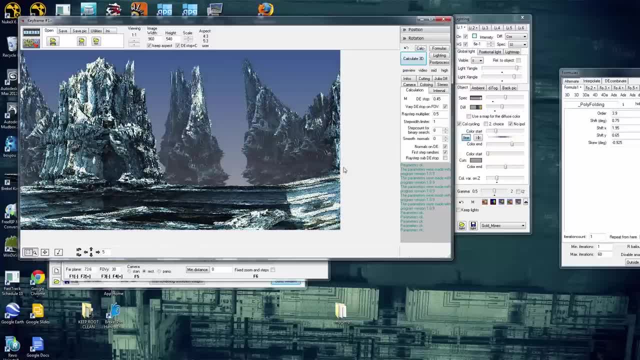 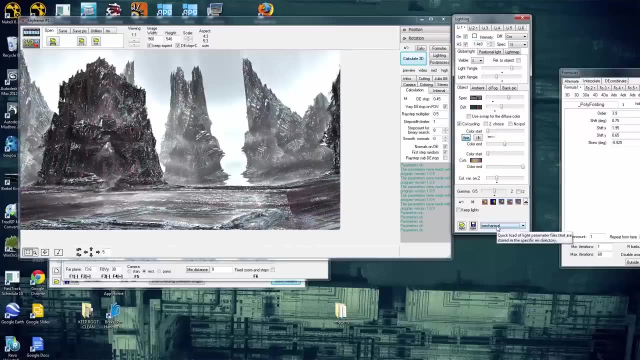 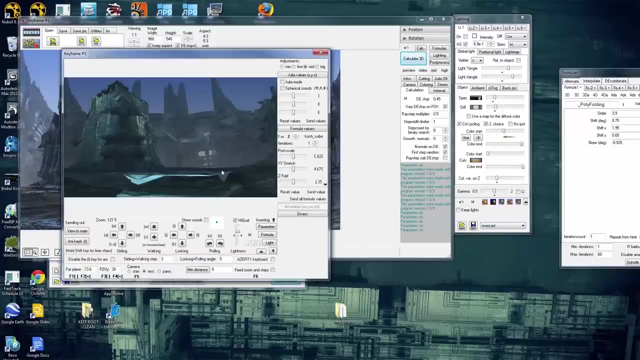 that can just blow people away with these fractals, and these are just some ways that i have thought about and that we have thought about at hectic electric. that can actually make this from something that you could do- if only you had the software- to something that you can actually say: we can actually do this. i'm julius, first house. i'm a visual effects. 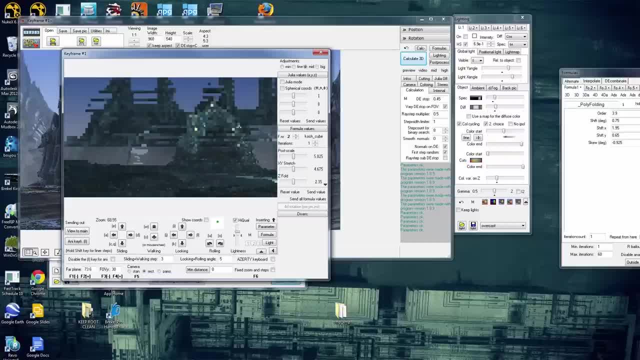 supervisor and a fractal artist for hectic electric in amsterdam, and i thank you very much for listening. bye. 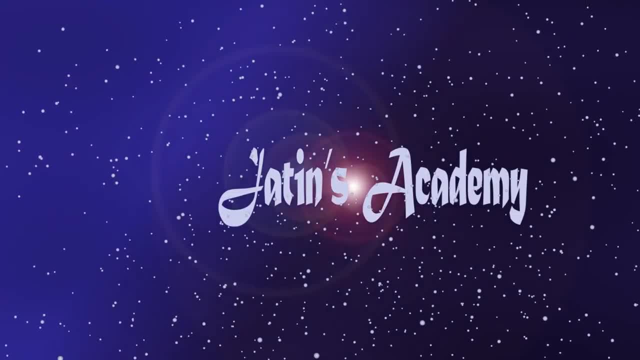 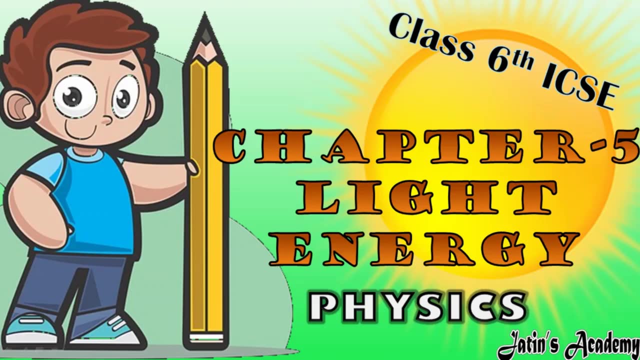 Good morning, dear students. Welcome to Jatin's Academy. So today, in this class, we are going to start with the fifth chapter of class 6, ICSC physics, that is, light energy. So in this class we are going to study first of all sources of light that is luminous and